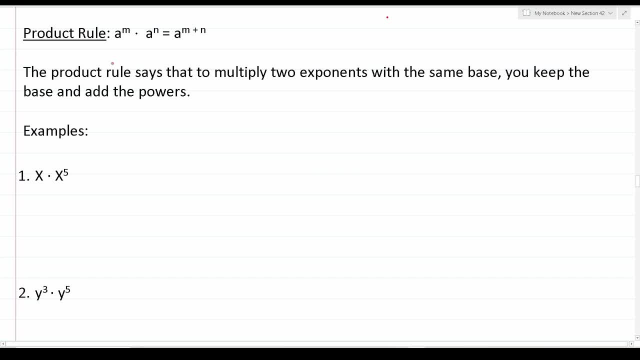 let's go ahead and quickly review how to do that Again. the product rule says this: To multiply two exponents with the same base, you keep the base the same and then you add the powers. So here you can see we have base a raised to the m power, Base a raised to the n power. 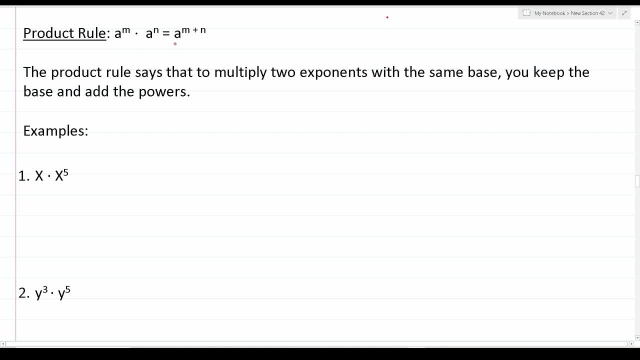 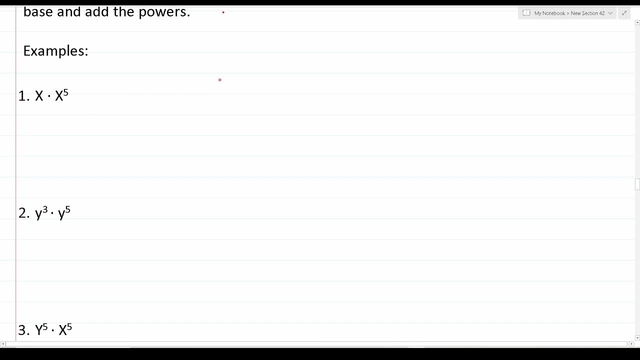 when we multiply those, since they have the same bases, we keep the base the same and we just add the powers. So let's go ahead and get some practice doing that before we move on to multiplying polynomials. and at this point in the video, if you want to pause the video and attempt, 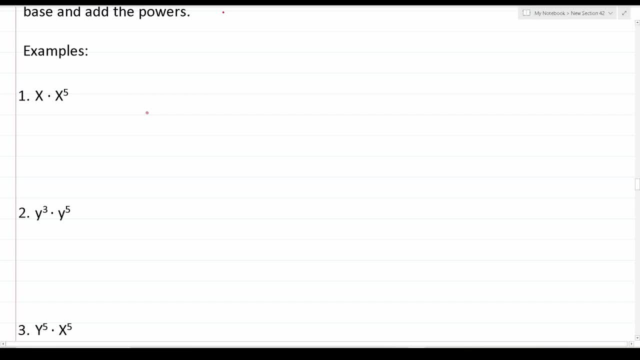 to work these out on your own. I'd encourage you to do so. otherwise you're more than welcome to just follow along. So this first question says x times x to the fifth. Well, I'm going to write this off to the side. over here again, we have x times x to the fifth In order to apply the product rule. 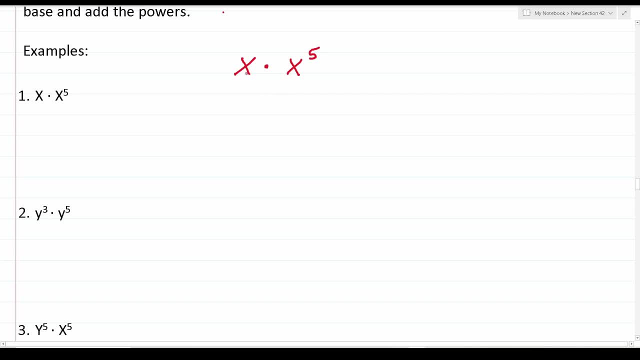 we have to have the same bases and in this case we have a base of x here and a base of x here, so we can apply the product rule here. That said, it may not be obvious that this x right here is raised to the first power. Again, when anything's raised to the first power, it's not going to be expressed. 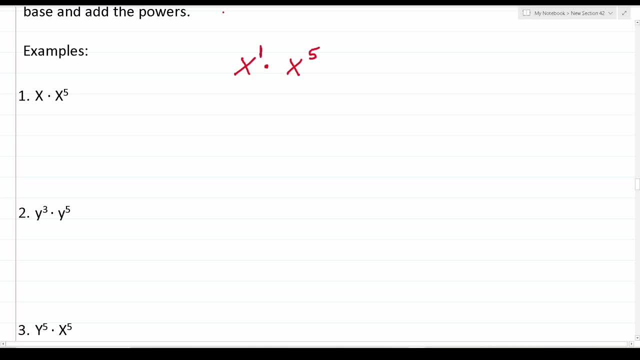 but, that said, if you're working this out, you can simply add that one there and then, according to the product rule, this is simply going to become x to the one plus five, which is the same as x to the sixth. Let me go ahead and put a box around that to indicate that this one is done. 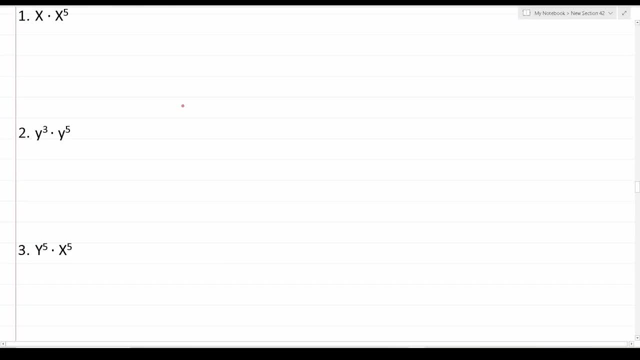 All right, let's take a look at example two now. In this case, we have y to the third times y to the fifth. We have y to the third times y to the fifth. Again, in order to apply the product rule, we have to ensure that the bases are the same. 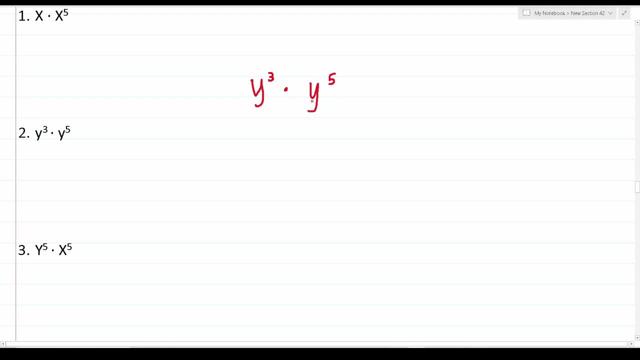 In this case, we have base y raised to the third power and base y raised to the fifth power. Since the bases are the same, we know our answer is going to look like this: We're going to keep a base of y and then we're simply going to add the exponents together. 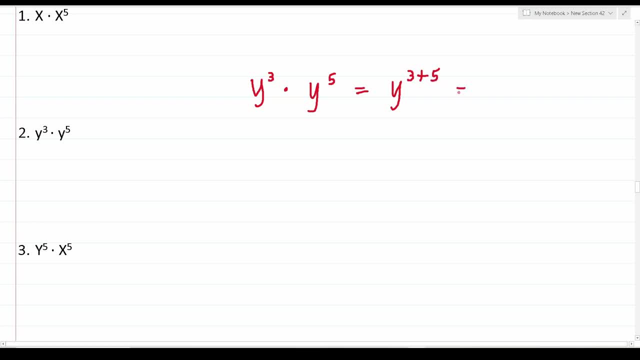 So this is going to become three plus five, and of course, three plus five is just eight. So in other words, y to the third times y to the fifth is y to the eighth. All right, let's go ahead and take a look at number three. now I'm simply going to 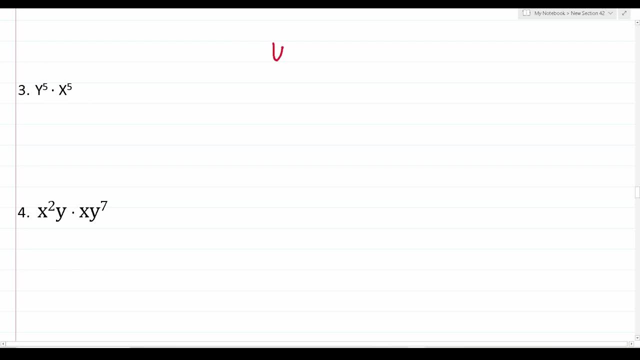 start by copying it off to the side here. So we have y to the fifth times x to the fifth. in this case we cannot use the product rule to combine the exponents because they don't have the same basis. Again, in order to apply the product rule, you have to have the same basis, Remember. 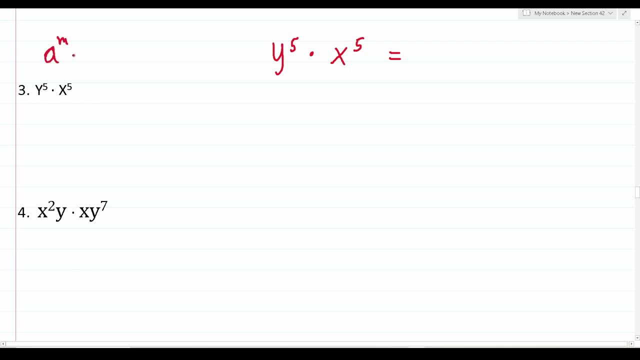 the product rule was: a to the m, times a to the n results in a to the m plus n. Again, look, the bases are both a. In this case we have a base of y and a base of x, so we can't combine their exponents. 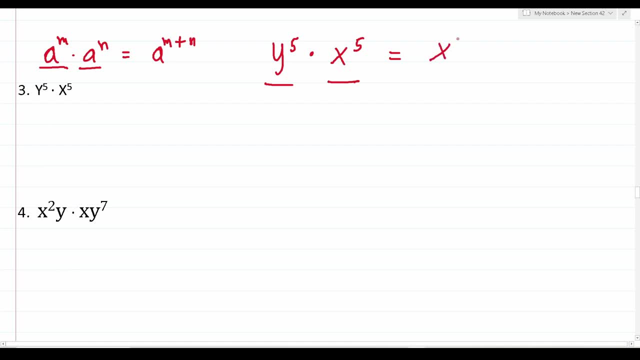 That said, we can rewrite this as this: x to the fifth times y to the fifth. That is to say, we can actually get rid of this multiplication sign just by combining these like this: All right, so that's that one, and let me put a box around it to indicate that we're done with it. And finally we have x. 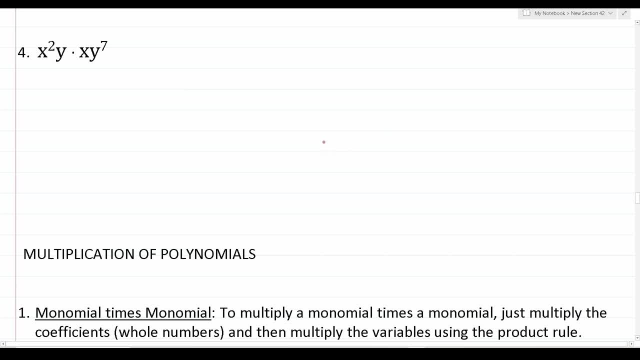 squared y times x, y to the seventh. So let's go ahead and copy this one off to the side. We have x squared y times x, y to the seventh. All right, so if it's helpful, wherever you don't see an exponent, you can fill in a one accordingly. And now we're going to apply the product rule, but we can only. 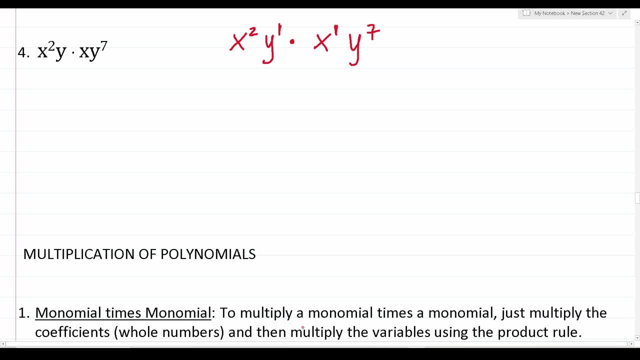 again apply the product rule to the variables that have the same basis. So first I'm going to apply the product rule with these x's, So this becomes x, and again we're simply going to add their exponents, So this is going to become x. 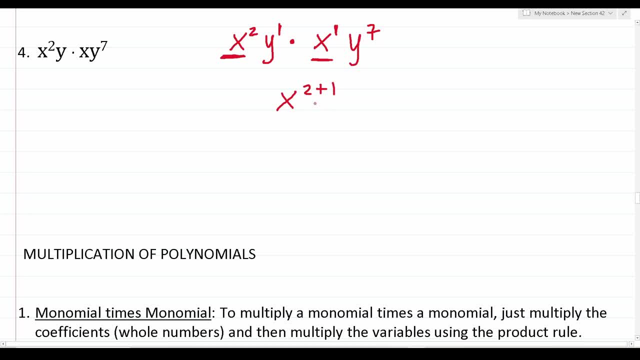 two plus one. And then, likewise, we're going to use the product rule to combine the exponents for the variables that have the base of y. So this becomes y one plus seven. And let's go ahead and do that simple arithmetic there. This becomes x to the third. 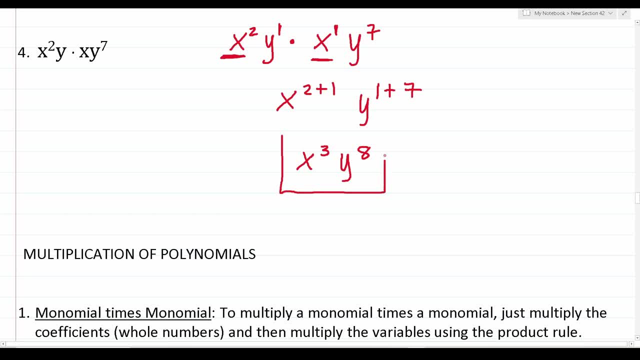 times y to the eighth. All right, so, as you're going to see in just a few minutes, many of the questions we're going to work with are going to be jumbled up like this. So again, just remember that, according to the product rule, you can only add exponents if the bases are the same. All right, so with that in. 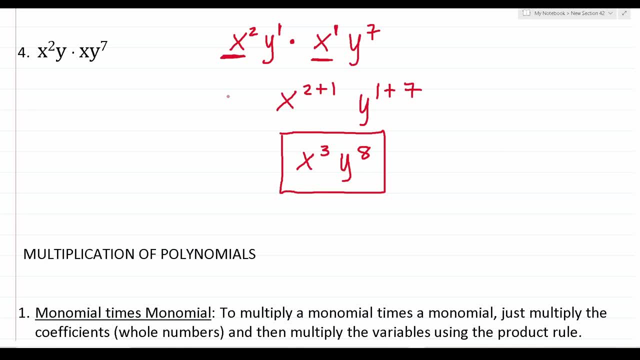 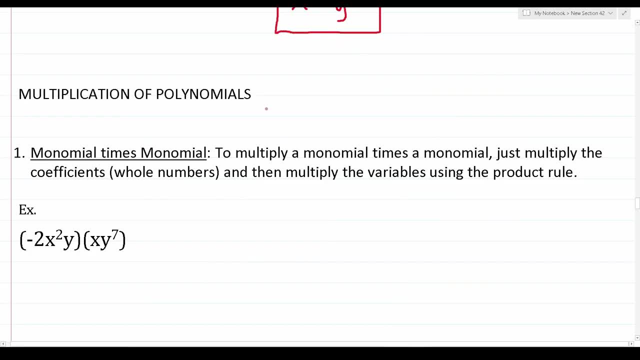 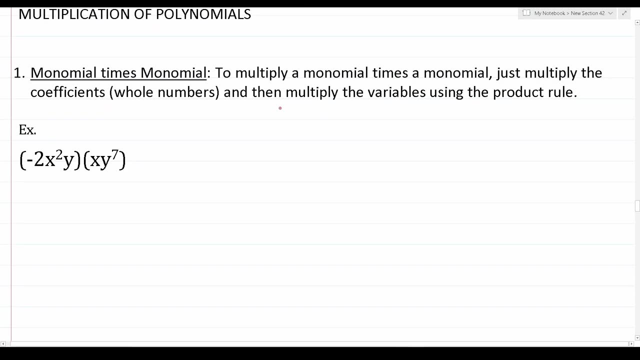 mind, let's go ahead and take a look at our first case of multiplication of polynomials. All right, so now that we've reviewed the product rule, let's take a look at a few examples involving the multiplication of polynomials. To start, let's look at the most basic instance of that. Notably, let's look at what happens when we 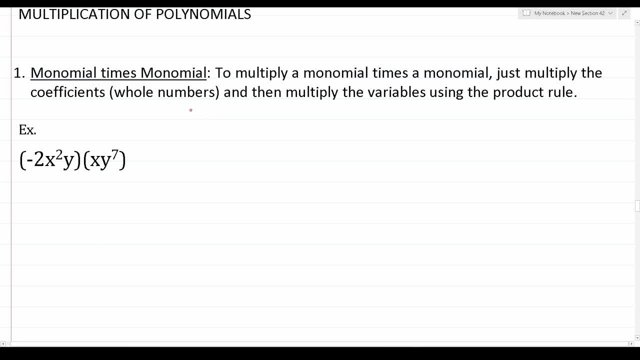 multiply a monomial times a monomial. And in case you forgot, a monomial is simply a polynomial that only has one term And, if you look right here, this is one term and this is a another term. So we're taking this monomial and multiplying it by that monomial, And I did define. 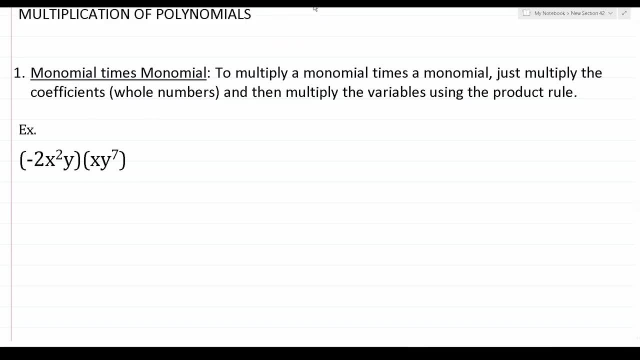 that in yesterday's video, so if you want to go back and watch that, that'd be a good idea. But that said, as far as multiplying monomials together goes, it says to multiply a monomial times a monomial, just multiply the coefficients, that is the whole numbers, and then multiply the variables. 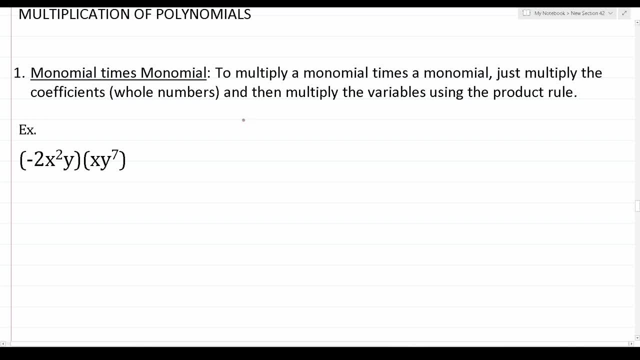 using the product rule. So let's go ahead and write this one off to the side. As you can see, we have negative two x squared y, and instead of using parentheses, I'm just going to put the multiplication symbol there. times x, y to the seventh: All right, so the first step is to take care of our 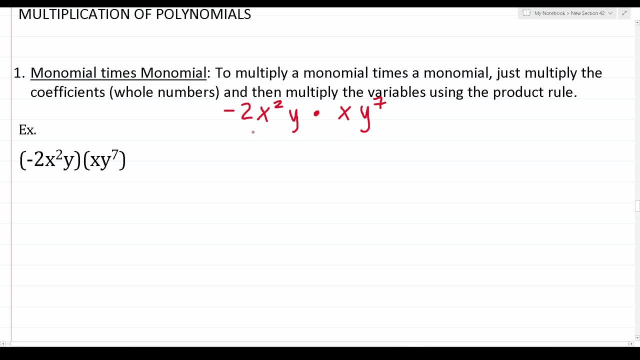 coefficients. So our coefficients are the whole numbers. We have a coefficient of negative two here. That said, what's the coefficient in front of x here? Well, whenever the coefficient is not expressed, it's implied that it's a one, And likewise we can go ahead and add our implied one. 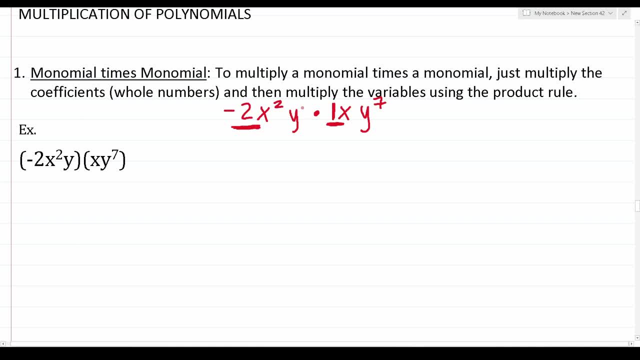 exponents as well. So again, there's no exponent on top of this y, so let's put a one there. and there's no exponent above this x, so it's implied that it's a one. All right, so let's take care of the coefficients. This becomes negative, two times positive, one Negative times, a positive is going. 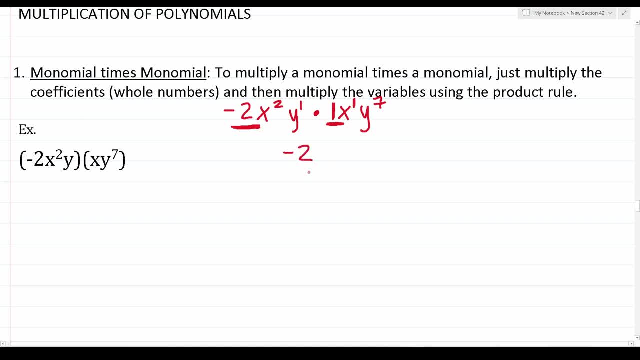 to be a negative, so this is just negative. two: Now, using the product rule, let's go ahead and take care of our variables. This says x squared times x to the one. Again, according to the product rule, we keep our base the same and then we add the. 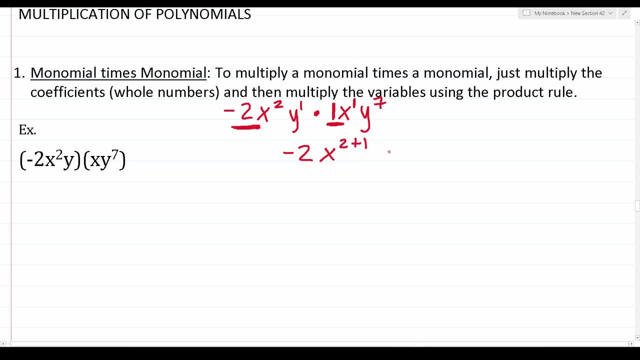 exponents. so this becomes x to the two plus one. Let's do the same thing here for y. Keep y the same and then add the exponents Again. this says y to the first times, y to the seventh, according to the product rule. that becomes one. 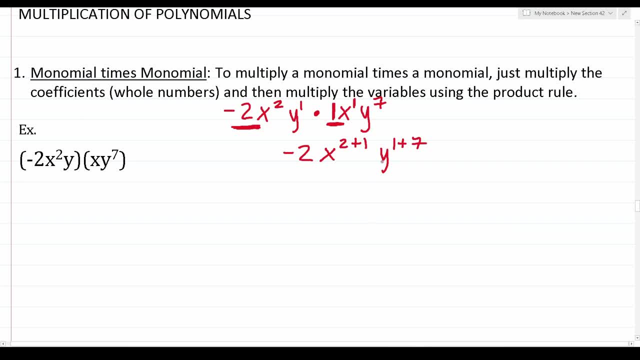 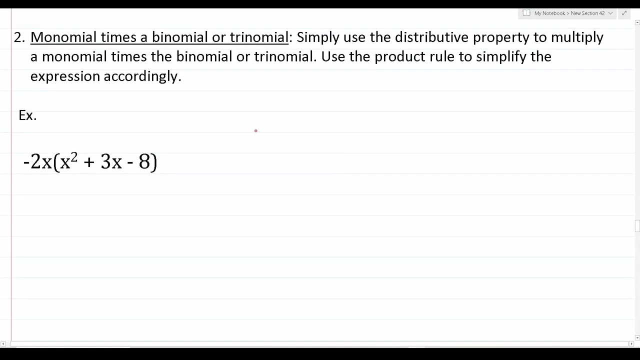 Plus seven. Let's go ahead and do this simple arithmetic to clean this up a little bit. We have negative two x. Two plus one is three, and then y. one plus seven is eight. All right, that's all there is to multiplying a monomial by a monomial, All right. so now that we've seen that, let's go. 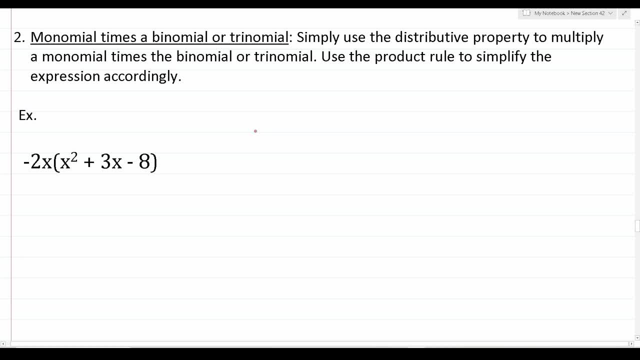 ahead and work on another instance involving the multiplication of polynomials, And in this case we're going to look at what happens when we multiply a monomial times a binomial or trinomial. Again, as we know, a monomial is a one-term polynomial, whereas a 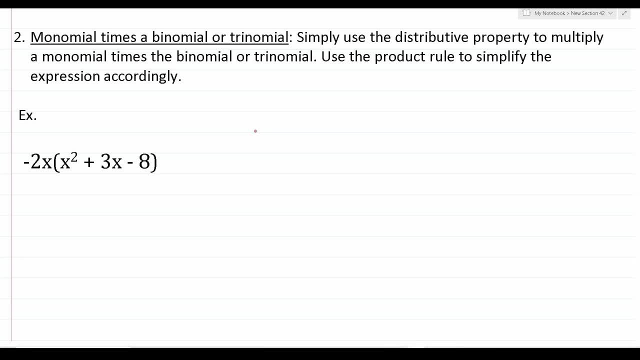 binomial is a two-term polynomial and a trinomial is a three-term polynomial And, if you like, following instructions. I went ahead and wrote out some simple instructions for you here. It says: simply use the distributive property of multiply a monomial times. 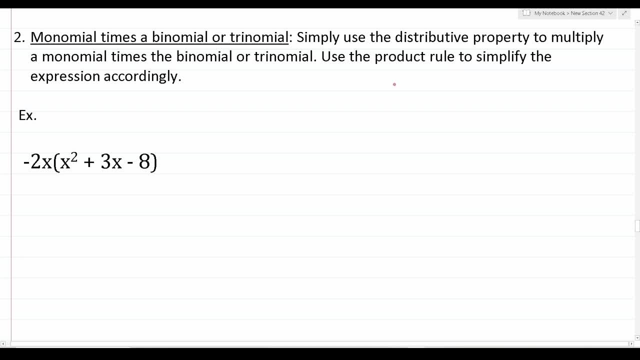 the binomial or trinomial and then use the product rule to simplify the expression accordingly. Let me just point this out: In this case, the term that's outside the parentheses is a monomial, since there's only one term, Whereas what's inside the parentheses is a trinomial, since there are three. 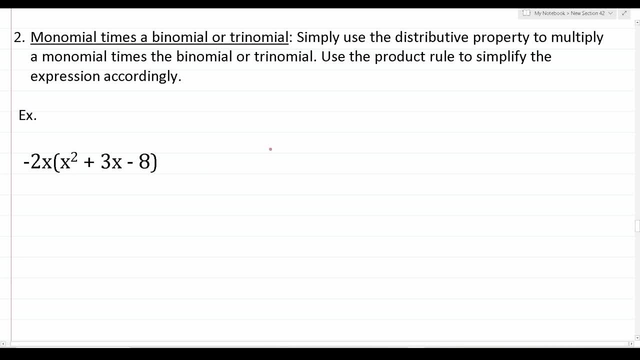 terms. Again, there's one here, one here and one here, So let me start this one by writing it off to the side. We have negative two x x times x squared plus three x minus eight. All right, so if it's helpful, you can go ahead and 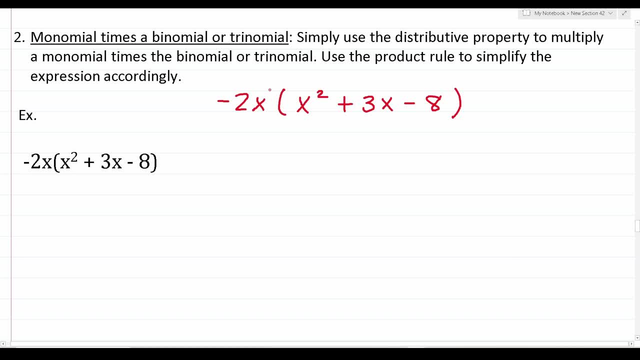 wherever there's not an exponent on a variable, you can place a one, since it's implied. And now that we've done that, we can go ahead and take this negative two x and distribute it here, here and here. So let's go ahead and see what that looks like. And again, 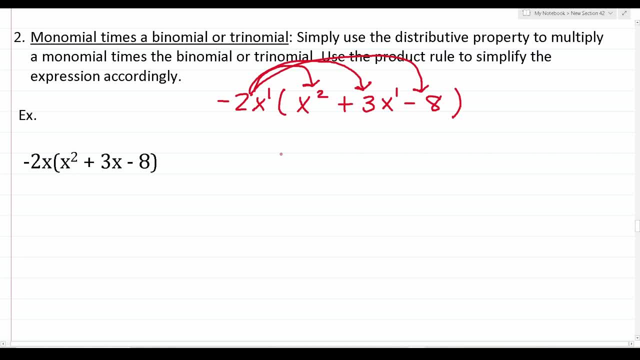 if you recall, when we multiplied a monomial by a monomial, it said: multiply the coefficients first. Well, if there's no coefficient, that means it's implied that there is a one coefficient there. So let's go ahead and expand this. We have negative two x to the first times, one x squared minus two beneficial primes. So that's one procedure. If I'm going to add one, that's going to be negative two x to the first times, one x squared minus three x minus eight. In this case, that's equal to negative two x the first times, one x squared. So we have two with two, one from the assets. That means we have two various shark under the axi. oh viene. So let's go ahead and expand this. When we型 Pauss, is it a similar three coefficient. so theging goes: andikka chang. And again here I put number two, and again, So put. 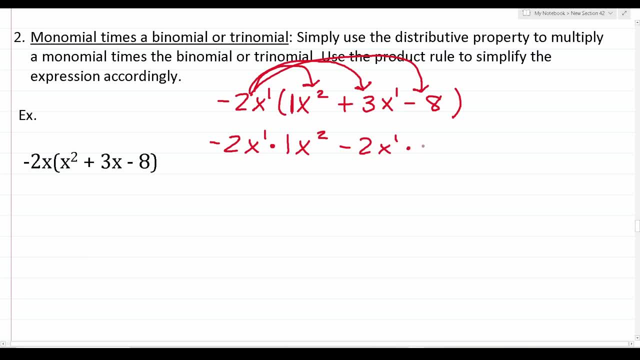 2x to the first times, 3x to the first, And then, finally, we have negative 2x to the first times, negative 8.. All right, now that this is expanded via the distributive property, let's go ahead and. 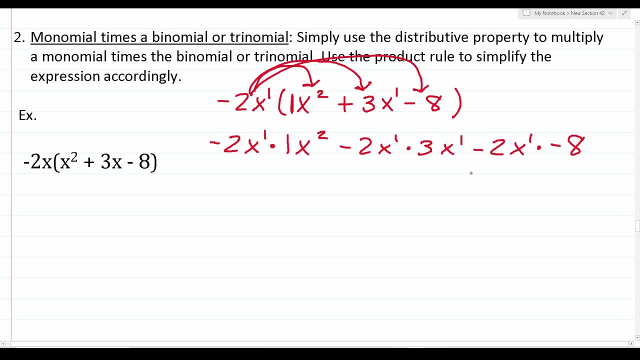 use the product rule accordingly to simplify this expression. So here we're just going to multiply the coefficients first, notably negative 2 and positive 1.. Negative 2 times positive 1 is going to be negative 2.. And then we're going to use the product rule to add these exponents. So 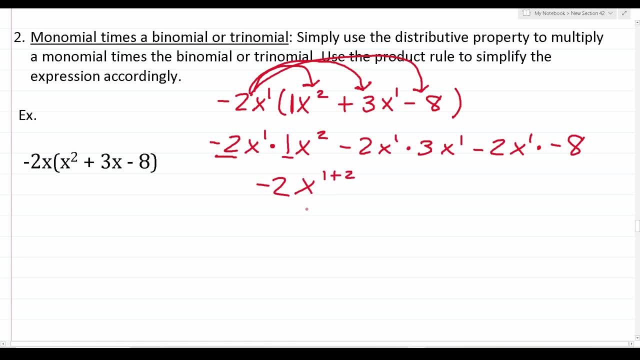 this becomes x to the 1 plus 2.. Right, here we're going to multiply our coefficients, notably negative 2 and 3. Negative 2 times positive 3 is going to be negative 6.. And then let's use the product rule. 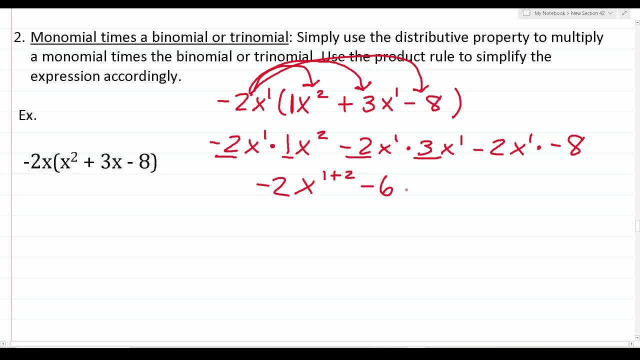 to deal with these exponents Again, we're just going to have x to the 1 plus 1 here, And then let's do this final one. now, Again, multiply the coefficients first, notably negative 2 and negative 8. And negative times, a negative 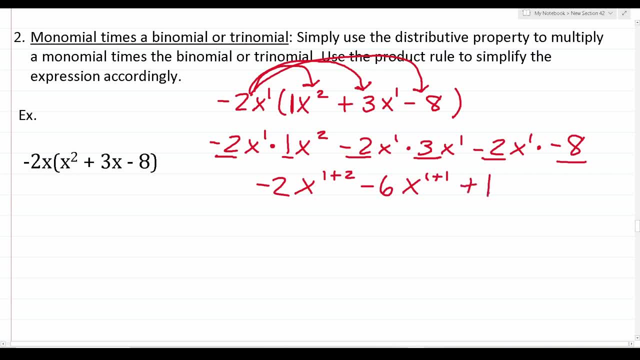 is going to be a positive, So this is going to become positive 16.. There's nothing to multiply this x by, So this just becomes x to the 1.. And now let's take care of these exponents, So this becomes negative. 2x 1 plus 2 is 3 minus 6x. 1 plus 1 is 2 plus 16.. Again, you don't express. 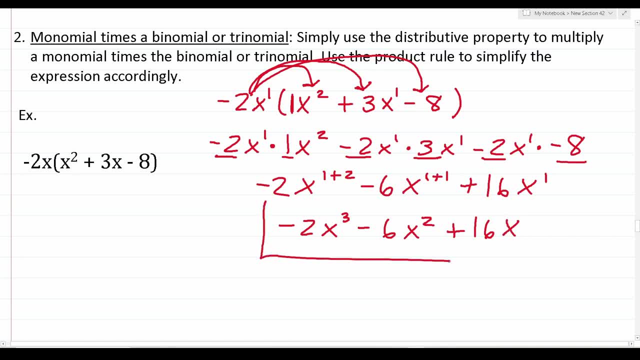 that 1.. So we'll just leave this as 16x And, just like that, we multiply this monomial by this trinomial. All right, So ultimately- and this is the reason I include a lot of practice questions in my video- 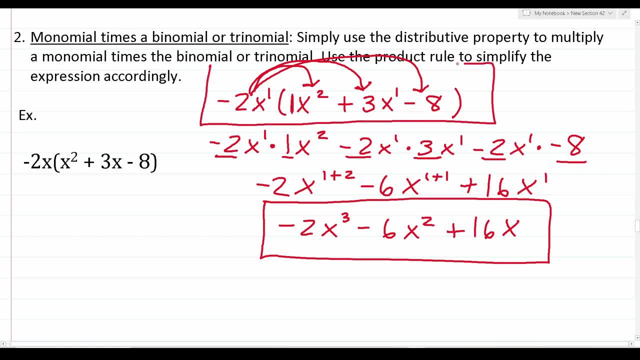 Ultimately, your goal is to be able to go from here right to your answer. Again, that's going to take a little bit of practice, But generally, once you get good at multiplying polynomials, you can look at one and go straight to the answer without having to write out these. 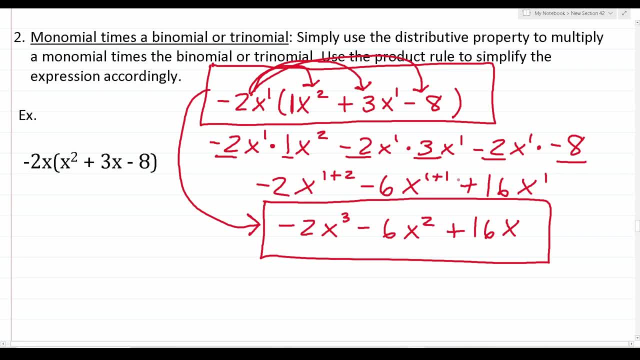 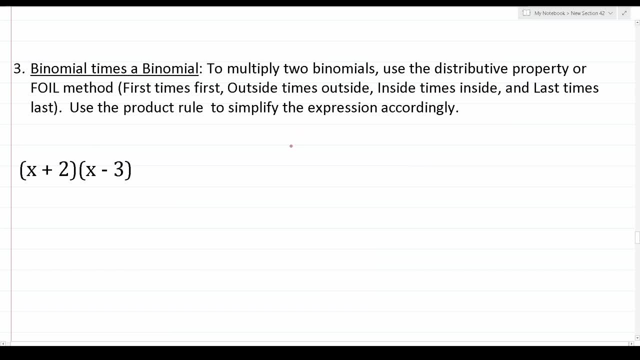 superfluous steps here. So, that said, let's go ahead and take a look at the next one. Let's look at another example, All right, So in this example, we're going to be multiplying a binomial by a binomial, That is, a two-term polynomial, by a two-term polynomial. And if 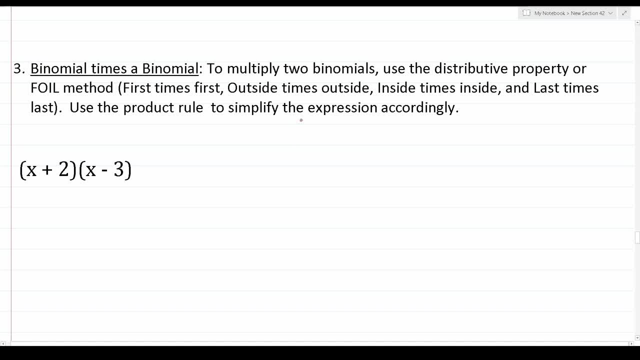 you like instructions, here they are. It says to multiply two binomials, use the distributive property or the FOIL method, And the FOIL method stands for first times, first, outside times outside, inside times inside and last times last. 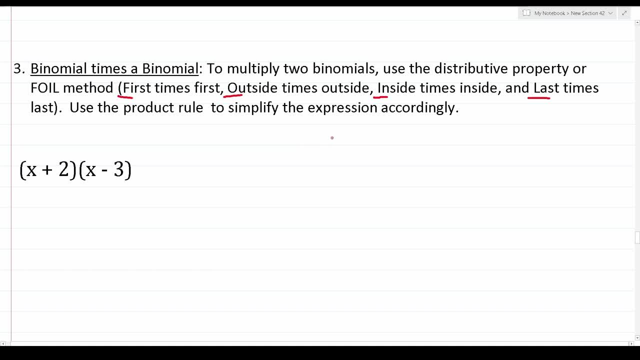 Once you do that, you're going to use the product rule to simplify the expression accordingly. Let me say this: I'm not a big fan of the FOIL method because, again, you're just using the distributive property. The FOIL method is just a name for the distributive property. 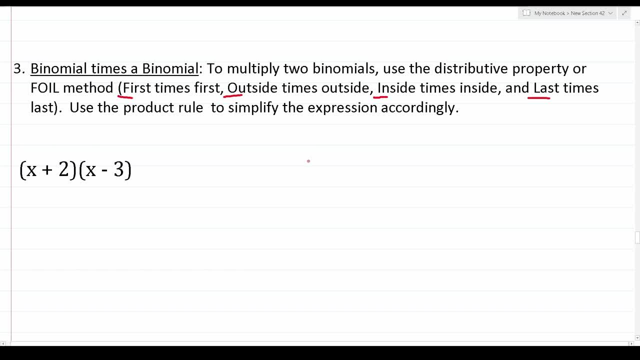 So let's go ahead and get started with this one. In this case, we have x plus two times x minus three times x, And, if it's helpful, you can go ahead and express the ones as your powers. where it's not present, Again, you don't have to do that, But that said, if you haven't done this in a while, 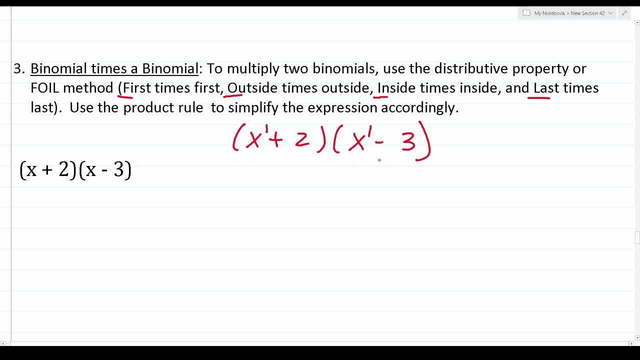 it might be helpful. This is x to the one, x to the one, And again, we're going to use the distributive property to expand this. And what that means is, to start, we're going to take this first term x and we're going to distribute it. So we're going to take this first term x and we're going to distribute it. 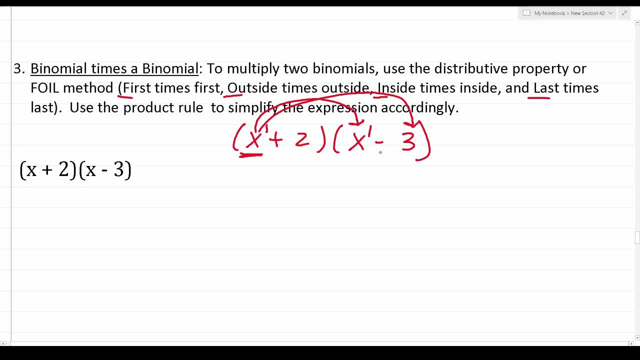 So we're going to distribute it here and here, And then we're going to take this second term two, and we're going to distribute it here as well as here, All right, so let's go ahead and get started doing that. So again. first we have x to the first times, x to the first. 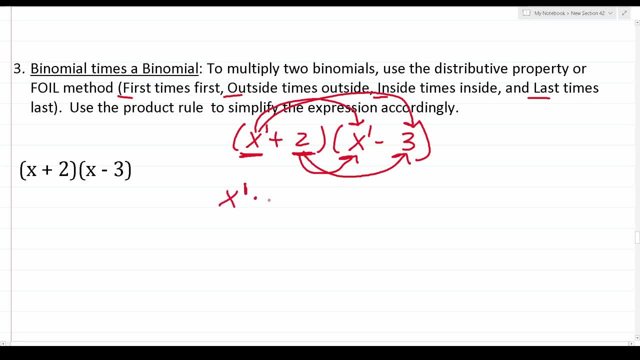 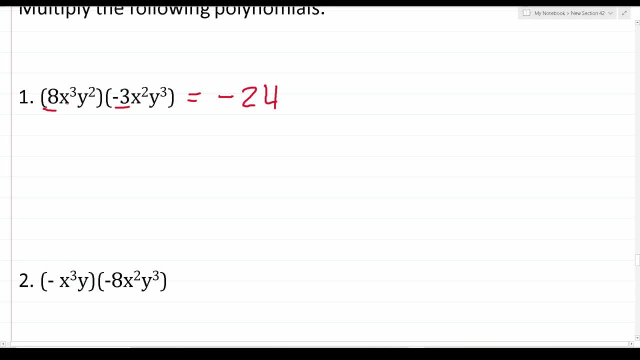 So that becomes x to the first times, x to the first. So that becomes x to the first times, x to the first exponents using the product rule, here we have x to the third times x squared according to the product rule. we're just going to add those exponents together, so this becomes x to the. 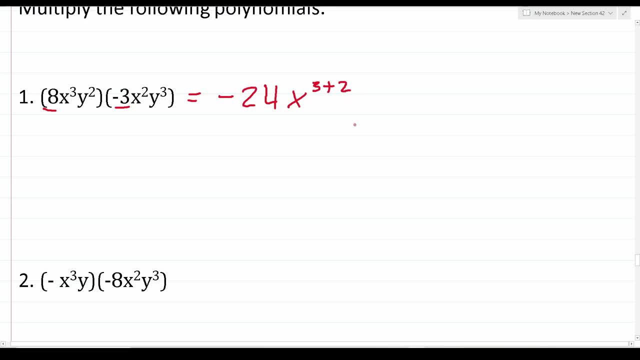 three plus two, and then finally we have y squared times, y to the third, again according to the product rule, we just add those exponents, so this becomes two plus three, and let's go ahead and simplify this a little bit further. this is negative 24. x to the fifth, y to the fifth. 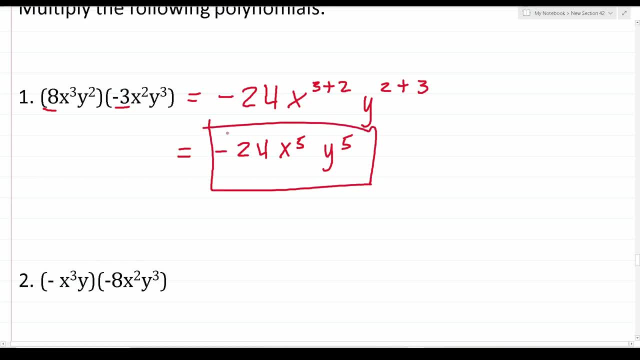 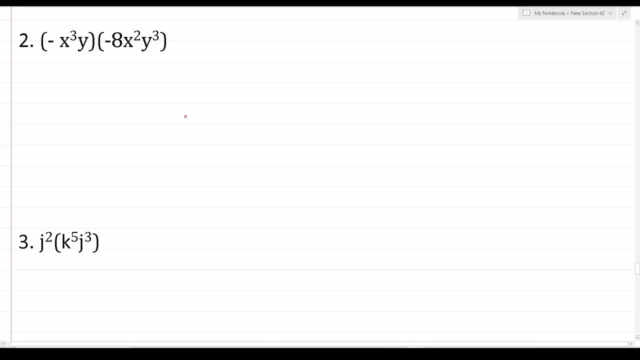 let me box that to indicate i'm done with that one. but nothing too difficult there. uh, number two says negative x to the third y times. uh, negative eight x, squared y to the third again. uh, there's an imaginary one here and there's imaginary one here. 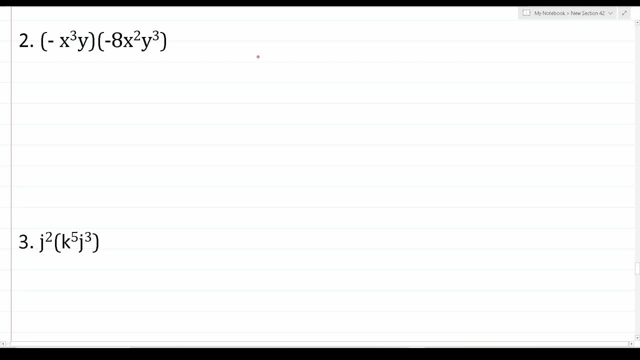 Here, I'm not going to express it Again. you want to get away from using those imaginary 1s and just work out the problem accordingly. So let's get started here. So we have negative 1, imaginary 1, times negative 8.. 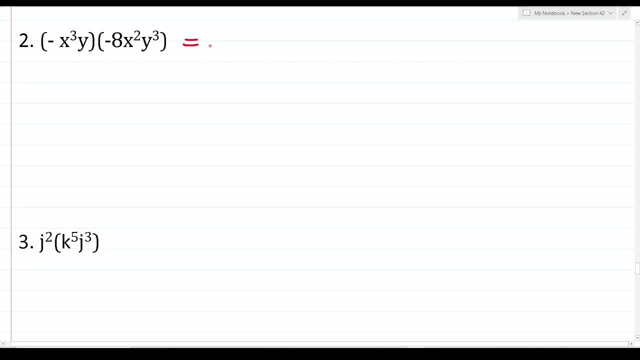 Well, negative times: a negative is going to be a positive And negative. 1 times negative: 8 is going to be positive, 8.. So our coefficients are done there. Now we're going to use the product rule to take care of our exponents. 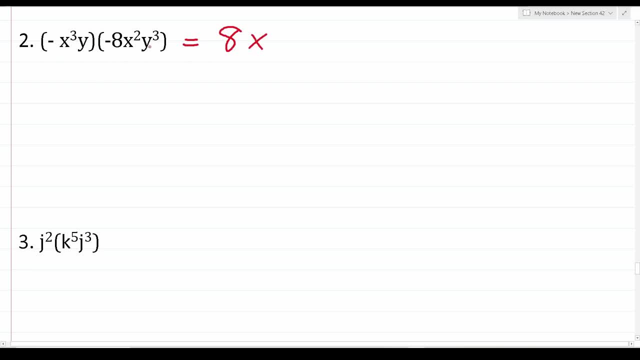 So we're going to look at our x's now. This is x to the third times, x squared Again according to the product rule. we just add those exponents, So this becomes 3 plus 2.. And now let's take care of our y's. 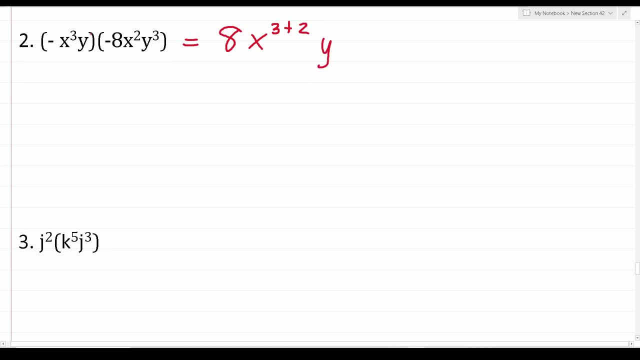 Again, there's an implied 1 here, So this is y to the first times, y to the third, According to the product rule. we're just going to add those, So this will be 1 plus 3.. Let's go ahead and simplify this a little bit further. 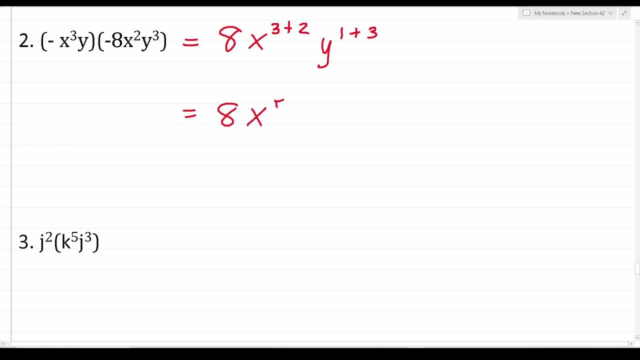 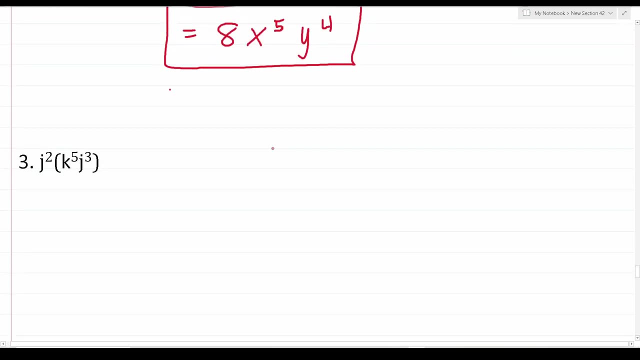 So this becomes 8x to the fifth, y to the fourth, And let's put a box around that one, since we're done with it. All right, So let's look at this next one, And I'm going to write it off to the side in case that's hard to see. 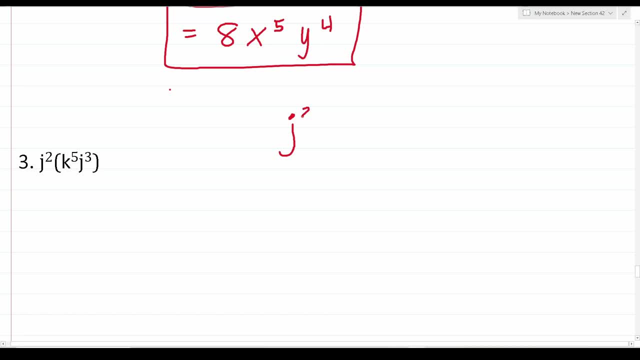 We have j Squared times, k to the fifth, j to the third- All right, So let's simplify this one Again. we can't really do anything with this j and this k, But, that said, we can use the product rule with j squared and j to the third. 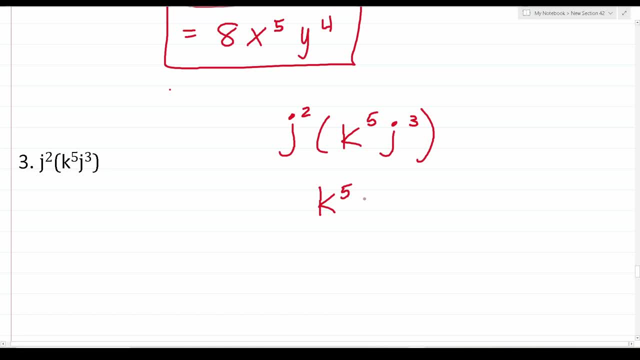 So this is going to become k to the fifth j, And then this is j squared times j to the third. According to the product rule, that becomes 2 plus 3.. So this simply reduces to k to the fifth, j to the fifth. 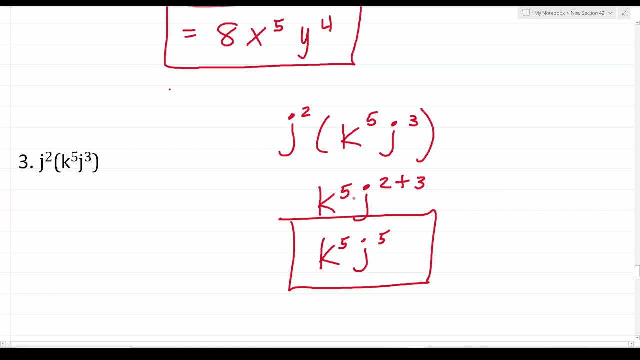 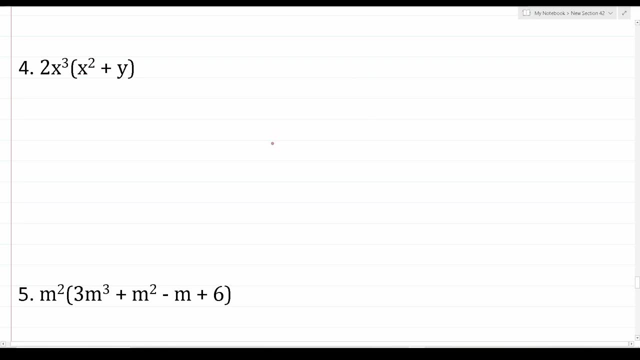 And we are done with that one. All right, Let's take a look at number four. now We have 2x to the third times x squared plus y in parentheses, So let me copy this one off to the side. We have 2x to the third times x squared plus y. 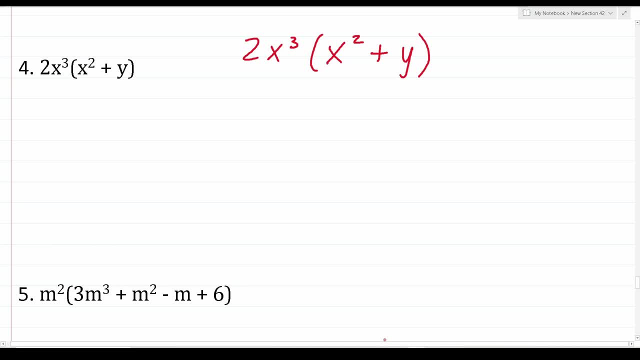 Again, we're going to have to use the distributive property to work this one out. That is to say, we're going to take this 2x, We're going to multiply it to this term And then, after we do that, we're going to have to multiply it to this term. 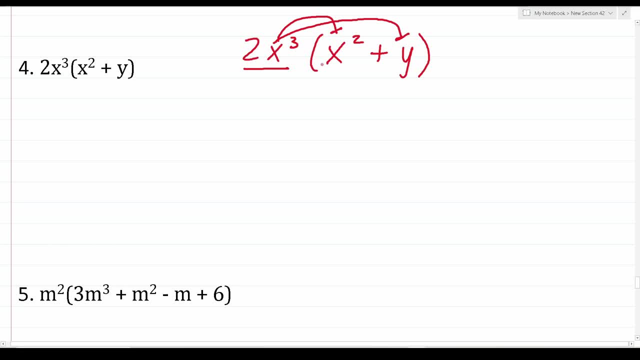 So let's go ahead and do that Again, if it's helpful. there's an imaginary one here. So this becomes 2x to the third, The third times x, squared plus 2x to the third times y. Let's clean this up a little bit. 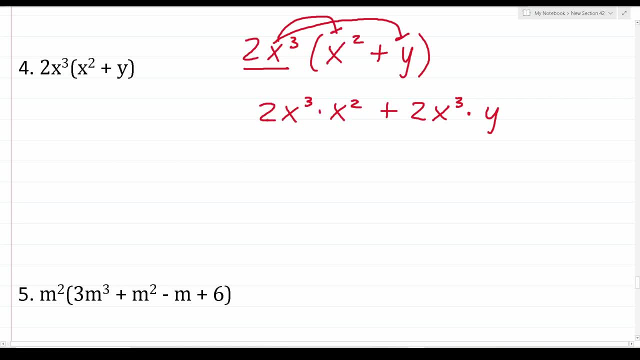 Again. first you look at your coefficients. This would be the same as 2 times 1.. 2 times 1 is just 2.. So this becomes 2x. According to the product rule. we can go ahead and add these exponents. 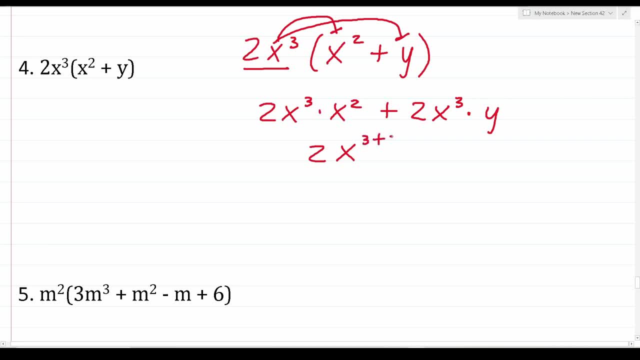 So this is going to become 3x, 3 plus 2.. And then this is plus, And there's nothing to do here except to get rid of this multiplication symbol by making this one term. So this becomes 2x to the third y. 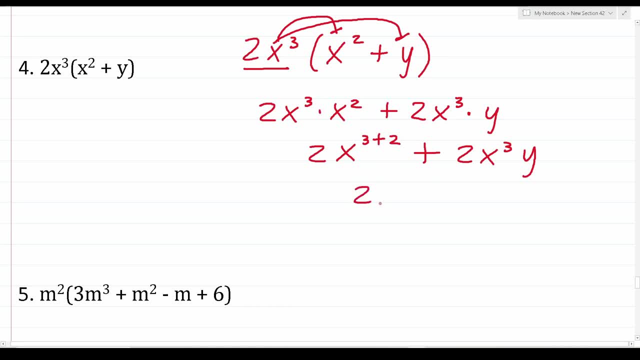 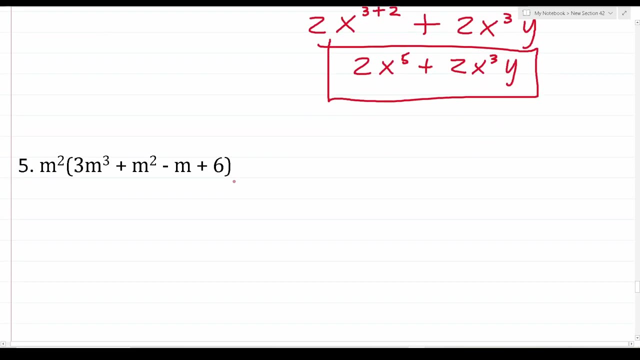 Let's go ahead and work this out very quickly. This is 2x to the fifth plus 2x to the third y, And just like that this one is done. Okay, All right, let's move on to number five now. 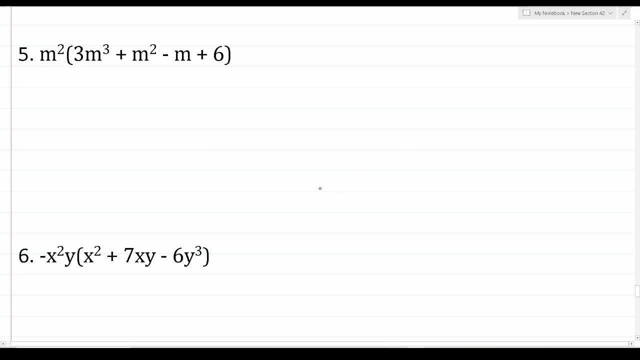 We're halfway done with this one, And for this one we have M squared times three M to the third, plus M squared minus M plus six. So I'm gonna copy this one down right here, So in case you're using your cell phone to watch this video. 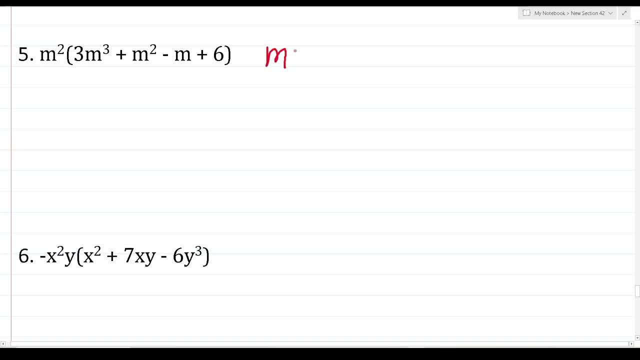 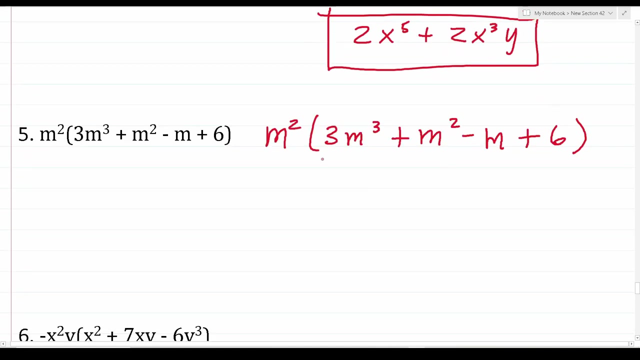 you can actually see it. So we have M squared three, M to the third, plus M squared minus M plus six. Again, we're gonna use the distributive property to take care of this one. More specifically, we're gonna take this M squared. 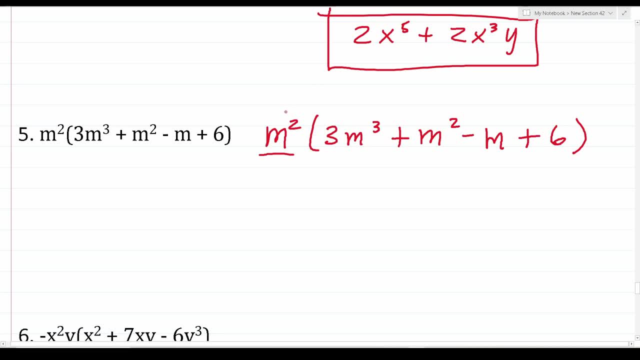 and we're gonna distribute it to every term inside the parentheses. So we're gonna take it, we're gonna multiply it here, here, here and finally here. It's kind of a tedious problem With that said, you will see stuff like this on the ASVAB. 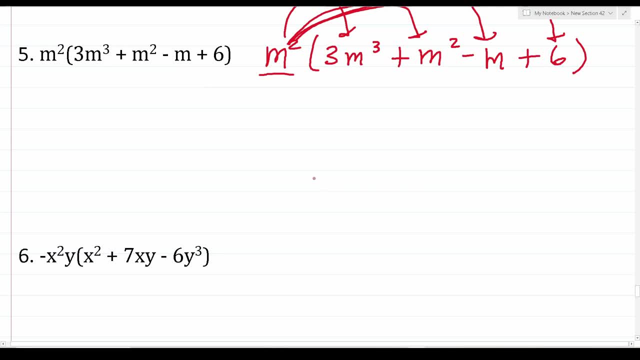 So better practice for it now than be caught flat footed on test day. So again, the first thing we're gonna do is M squared times three M to the third. Let me go ahead and express that over here. This becomes M squared times three M to the third. 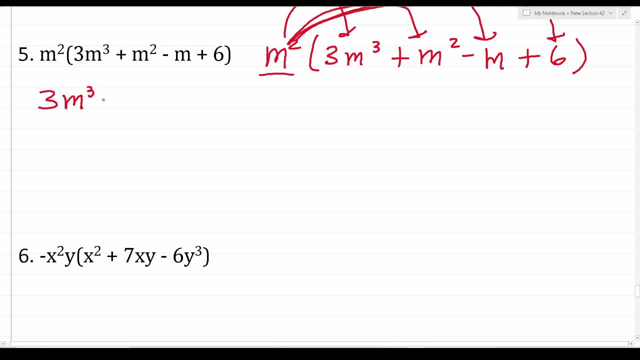 This becomes M squared times three. M to the third Times M squared. Then we have plus M squared times M squared, plus M squared times negative. M plus M squared times six. All right, let's use the product rule to simplify this. All right, let's use the product rule to simplify this. 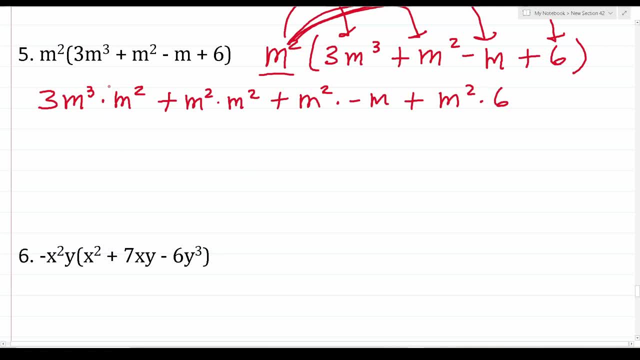 this one. accordingly, Right here there's a coefficient of one. So three times one would just be three. So this is three, And then, according to the product rule, we can add these exponents- So this becomes m, to the three plus two, plus again we can use the product rule. 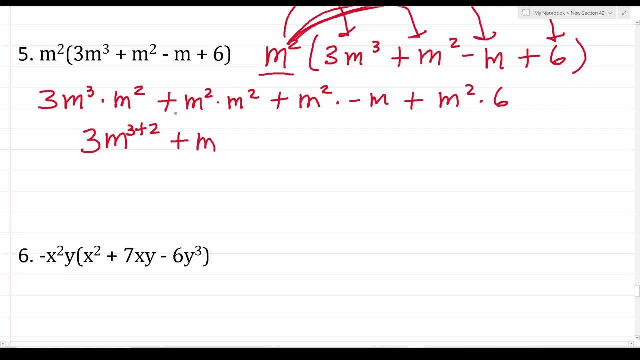 here. This will become m Again. there's a one here and a one here. One times one is just one, So that coefficient is just going to be one, And then this is going to be two plus two according to the product rule, And let's go ahead and work on this And let me get rid of that plus. 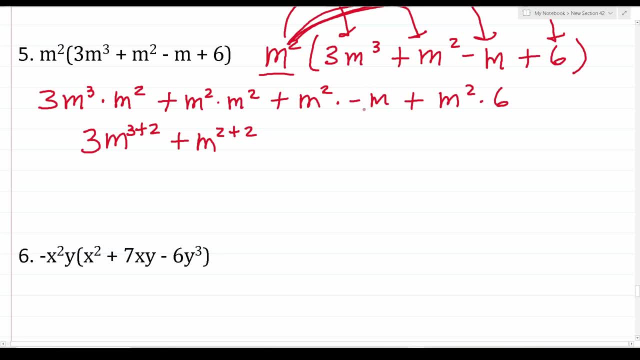 because again, there's an imaginary plus one here and an imaginary negative one here. Positive one times negative. one is going to be negative, So this is going to become negative m to the two. And again, what's right here? since it's not expressed, there's a one, right. 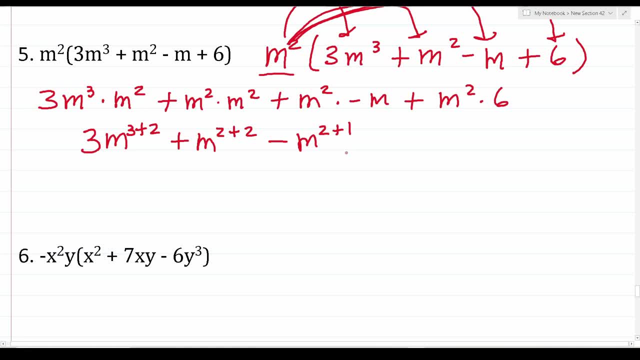 there. So that becomes negative m to the two plus one. And then finally we have this six times m squared. No product rule to use, but we can get rid of this multiplication sign. More specifically, we can write this as six m squared. All right, let's go ahead and simplify this now. So we have: 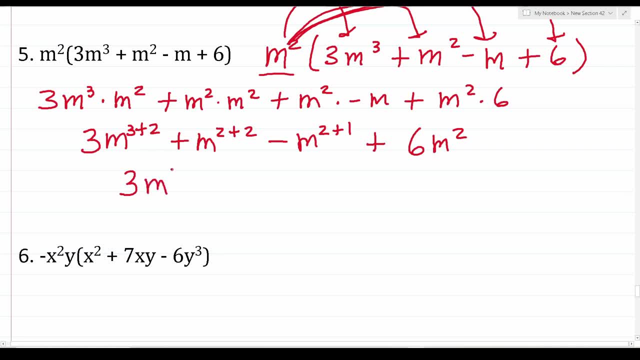 three m to the fifth, Plus m to the fourth, minus m to the third, plus six m squared. And you should notice this: When you're expressing these polynomials, you write them such that the terms with the highest powers come first. So here we have a power of five. You write that before any other power. 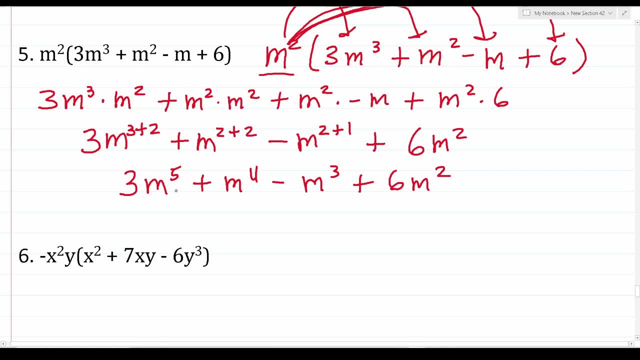 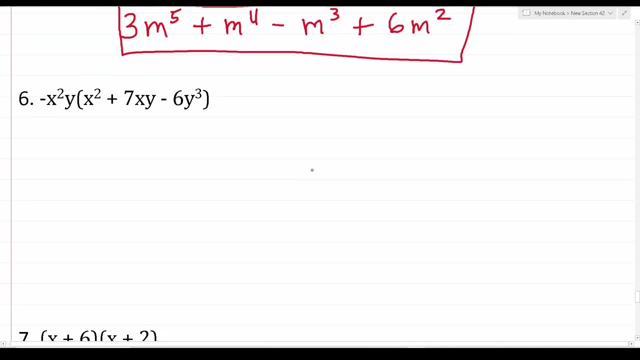 And then we have a power of three, And then we have a power of four, And then we have a power of two. So again, when you write these polynomials, the highest order powers come first, And you can see that that is the case in this one. We go five, four, three, two. All right, let's look at number. 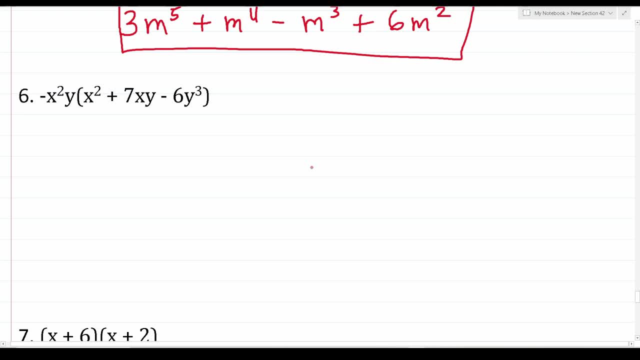 six. now Number six is a little bit challenging, But the same idea. we have negative x squared y times x squared plus seven, x, y minus six, y to the third. Again, we're going to use the distributive property first, which means we're going to take this first term and distribute it. 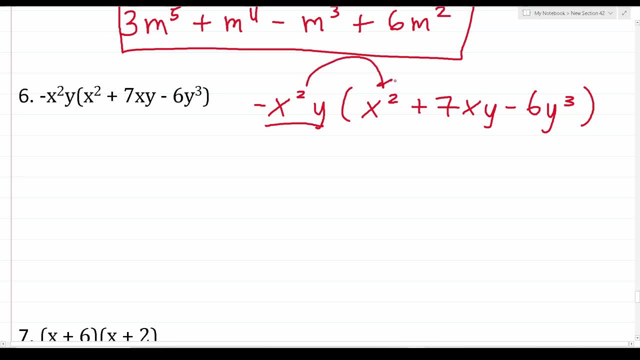 to everything inside parentheses. So we're going to take it and distribute it here, here and finally here. So let's go ahead and work on this And we're going to take this first term and on doing that, Again, I'm not going to express those implied ones. But that said, as you can see, 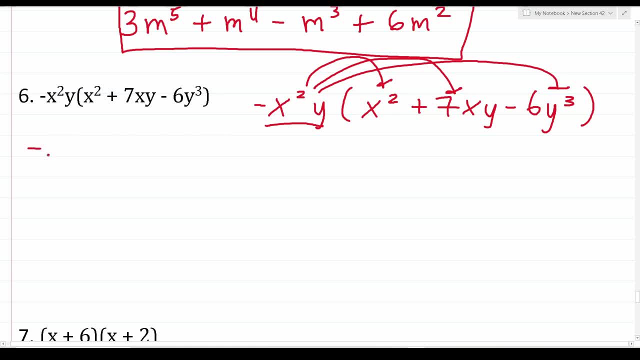 the first thing we're doing is we're taking negative x squared y and we're multiplying it by x squared. After that, we're taking negative x squared y and we're multiplying it by seven x- y. And then, finally, we're taking negative x squared y and we're multiplying it by seven x y. 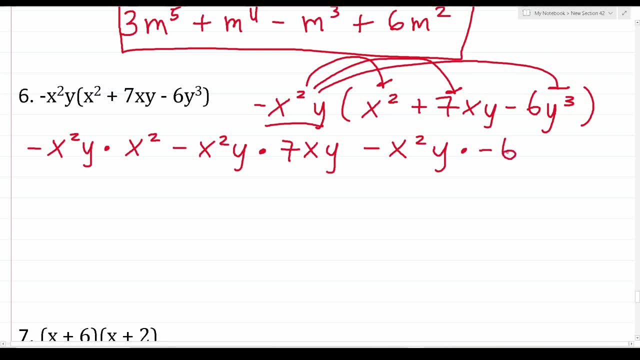 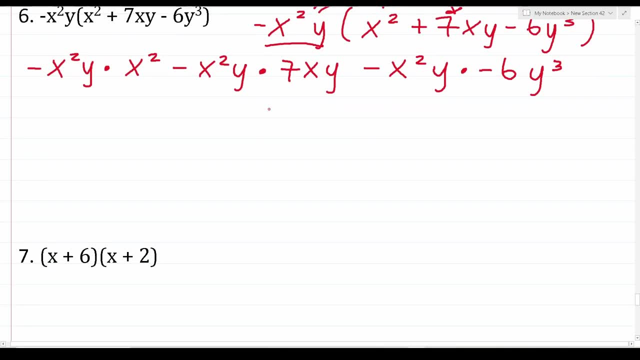 And we're multiplying it by negative six, y to the third. Let's go ahead and clean this up by taking care of our exponents as well as our coefficients. So again, technically, there's a one here and a one here. negative, one times negative. negative one times positive. one would be negative one, So we're. 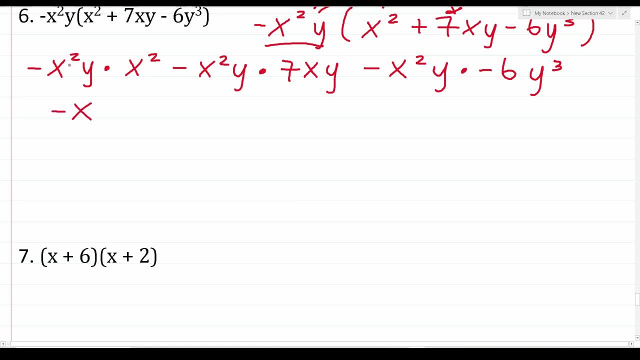 just going to leave this as negative x. But that said, according to the product rule, we can add these two exponents such that they become two plus two, nothing to multiply y by. So we'll just leave that as is, Again, technically. 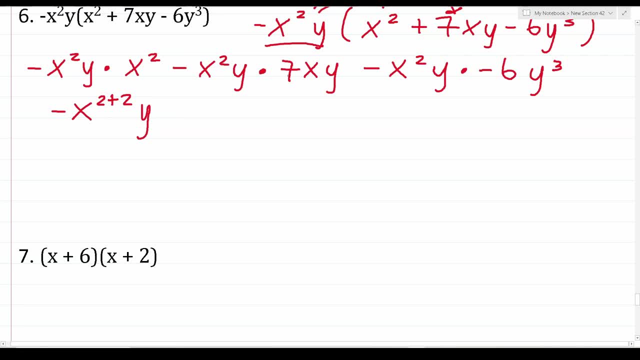 there's a one here. So this would be negative one times positive seven. So that's, that's going to become negative seven. Let's take care of the exponents now. starting with the x's, This becomes x. To that two plus one. Again, that one's implied there, And then we have y, and then this is one. 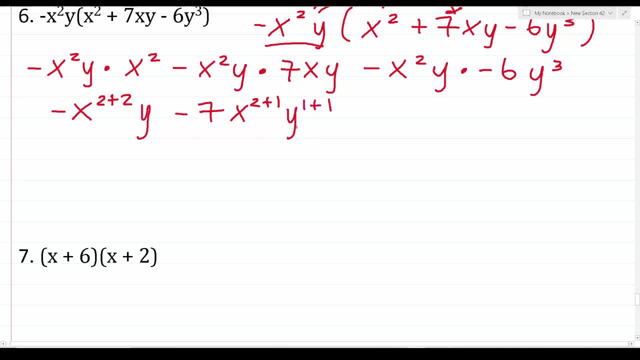 and one. So that's one plus one. Let's take care of this right. here we have negative x squared y times negative six y to the third. Again, technically there's a one here. So we have negative one times negative six and negative times. a negative is a positive, So this becomes: 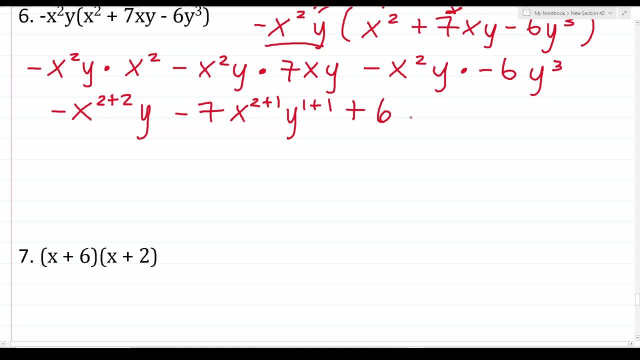 plus six, And let's take care of the exponents. now. There's nothing to multiply this x by, So this is just x squared. That said, we can apply that product rule here. So this becomes y to the one plus three. Again, that one's implied, right there. Let's go ahead and clean this up. Now this becomes: 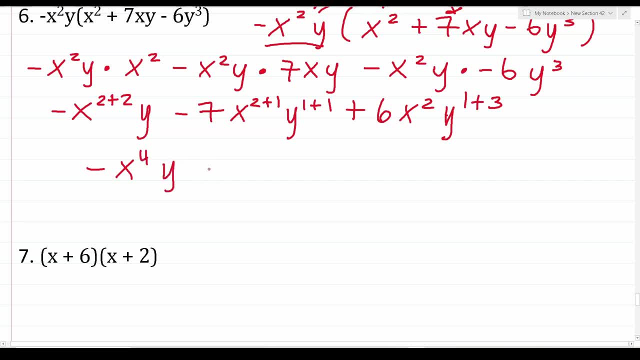 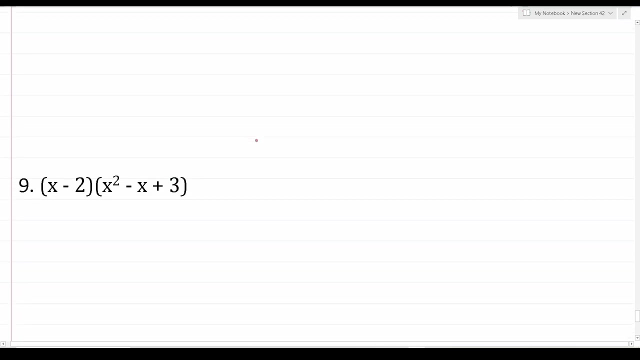 negative: x to the fourth, y minus seven, x to the third, y Plus six, x squared y to the fourth. Alright, so that is that one, And let's go ahead and move on to the next one. now, Thankfully, the next few are a little bit simpler. 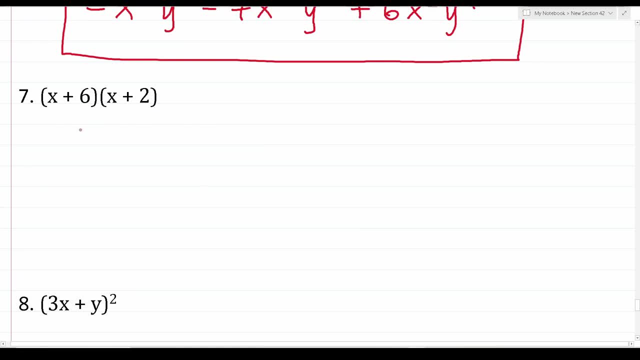 And, as you can see, we're multiplying a, a binomial, by a binomial. So we're going to take this first term, multiply it by both of these terms, and we're going to take this second term and multiply it by both of these terms, That's. 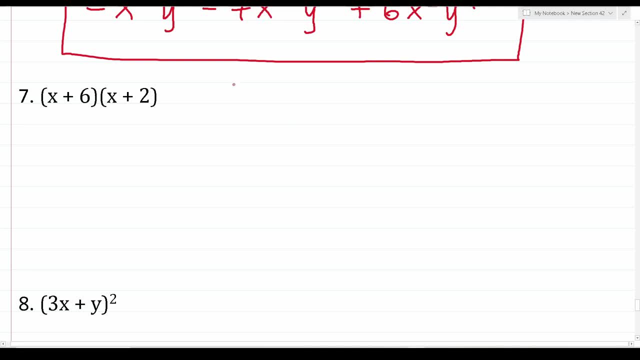 also called the FOIL method, if that's how you learned how to do that. That said, let's write this one off to the side. We have x plus 6 and x plus 2.. All right, so again we're going to use. 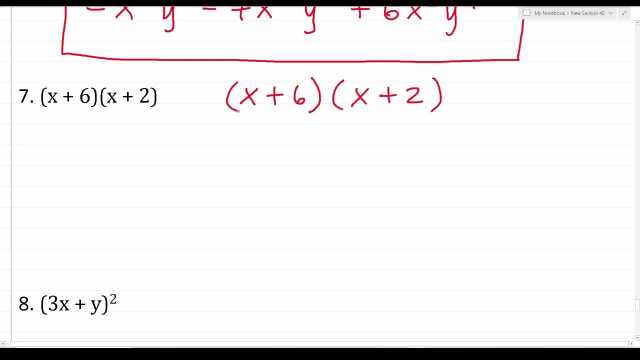 the distributive property to expand this one. So we're going to take this first term and multiply it by both of these terms. Then we're going to take this second term and multiply it by both of these terms. So let's work this out. This becomes x times x and then x times 2.. So plus. 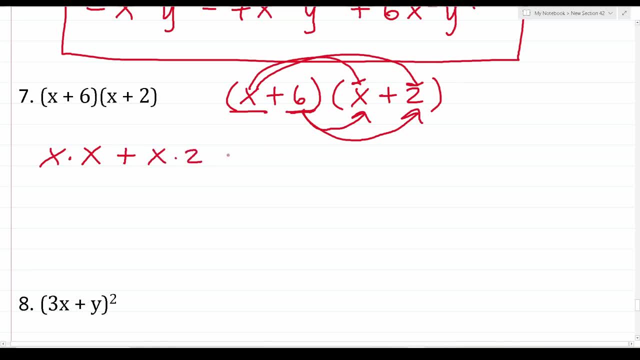 x times 2.. Now we're on to the sixth. This becomes plus 6 times x, plus x times 2.. Six times 2.. All right, let's go ahead and simplify this using the product rule, where applicable. So again, imagine there's these 1s here. This becomes x to the 1 plus 1.. 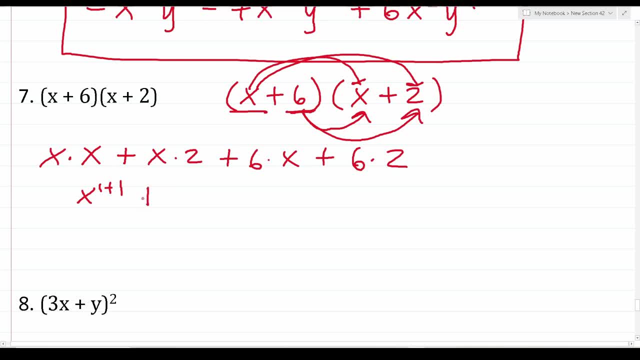 This just becomes x times 2,, which is the same thing as 2x. This becomes 6 times x, which is the same thing as 6x, And then this is just 6 times 2. Which is 12.. All right, let's clean this up now. This is x squared, And 2x and 6x are like terms. 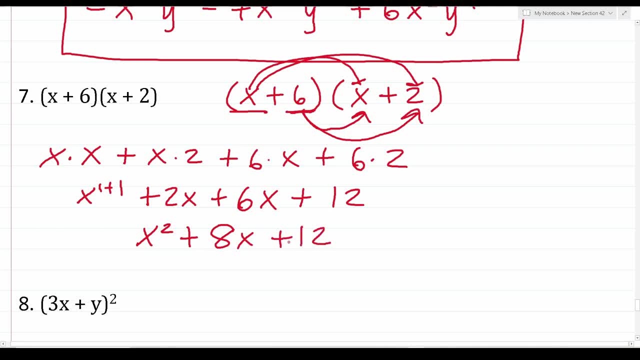 so we can add them. So this becomes 8x plus 12.. All right, so that's that one And again, you could have pretty much gone right from this to this, And if you were to go back to, if you keep practicing, you will be able to go from this right to your answer for these. 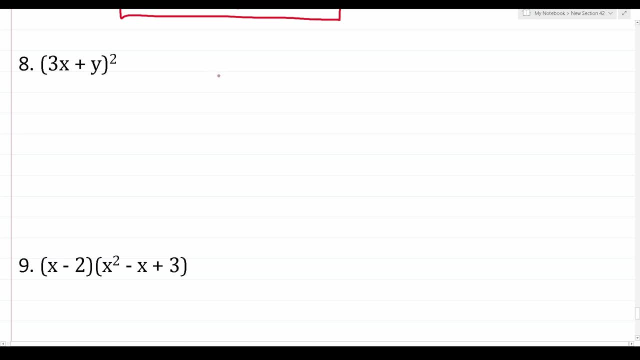 So, as we can see, number 8 says 3x plus y squared. Let's rewrite this so it's a little bit easier to work with. 3x plus y squared is the same thing as this: 3x plus y times 3x plus y, And here you can. either use the FOIL method or simply distributive properties. So 3x plus y squared is the same thing as this. All right, so we can use the FOIL method or simply distributive properties. So 3x plus y squared is the same thing. 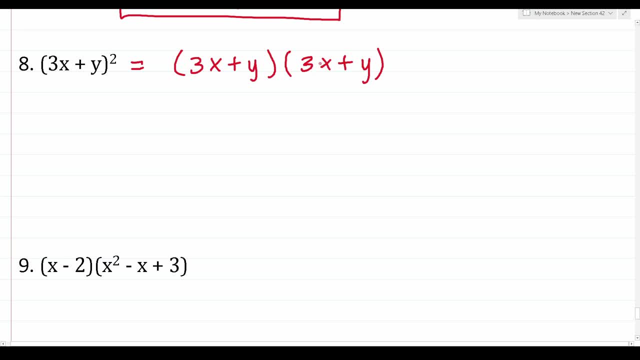 Again, I like the distributive property, which means you're going to take this first term and multiply it by everything in the second set of parentheses. So you're going to multiply it here and here. Then you're going to take this second term and multiply it here as well as here. So let's go. 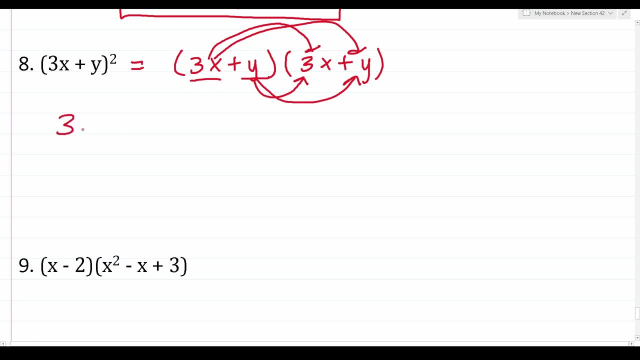 ahead and do that. As you can see, we have 3x times 3x, And then after that we're going to multiply by the second set of parentheses. So 3x plus y squared is the same thing as this. 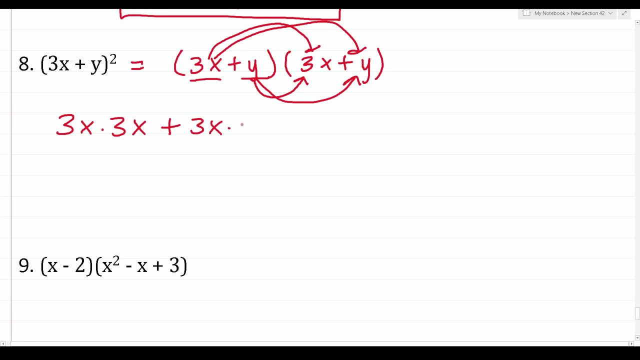 have plus 3x times y, and then we're going to move on to our y, so this becomes plus y times 3x, and then, finally, we have just y times y. So let's go ahead and start simplifying this Again. multiply your coefficients here, so this: 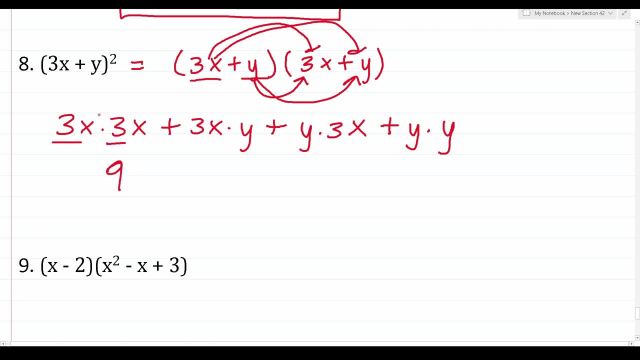 becomes 3 times 3, which is 9.. Again, those are. there are implied ones here, so we can use the product rule. this becomes x to the 1 plus 1.. 3x times y is just the same thing as 3xy, and that's all we have here. we have y times 3x, so this: 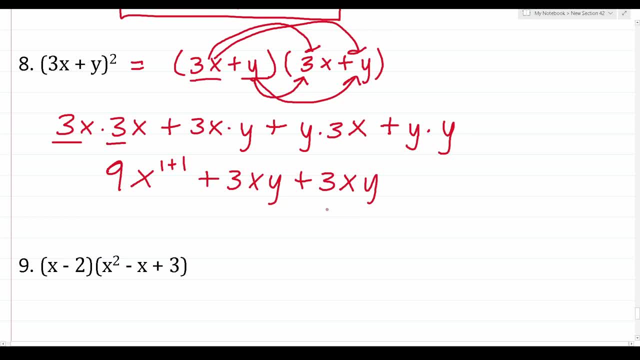 just becomes 3xy, and then here we can apply the product rule, since there are implied ones there. so this becomes y to the 1 plus 1.. Let's go ahead and clean this up. so this becomes 9x squared 3xy and 3xy are: 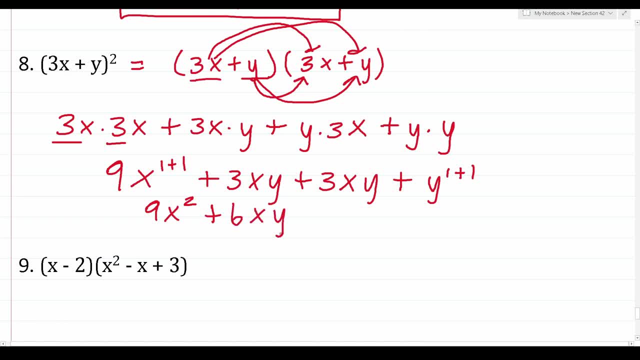 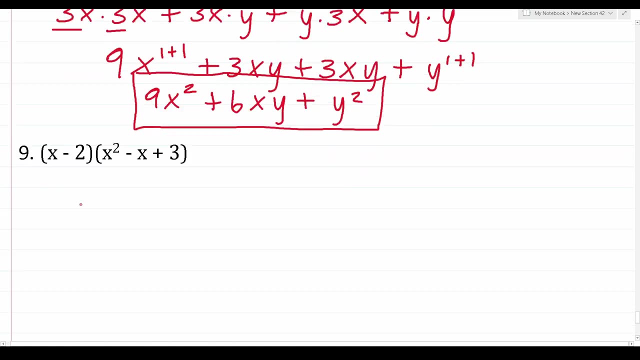 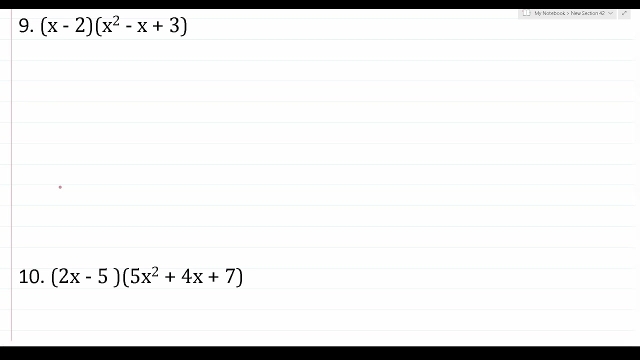 like terms. so this becomes plus 6xy, and then plus y, 1 plus 1, so that's y squared, and just like that we are done with this one. All right, two more to go. let's go ahead and start simplifying this. Let's go ahead and take care of them. for number 9, it says x minus 2 times x squared, minus x plus 3. so we're going to take both terms in this first set of parentheses and distribute it to all the terms in the second set of parentheses. 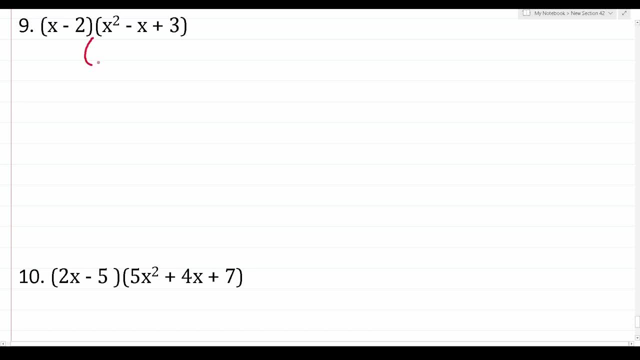 So let's see what that looks like again. we have- and let me go down a line here we have x minus 2 times x squared minus x plus 3.. All right, so we're going to take this x and distribute it here, here and here. 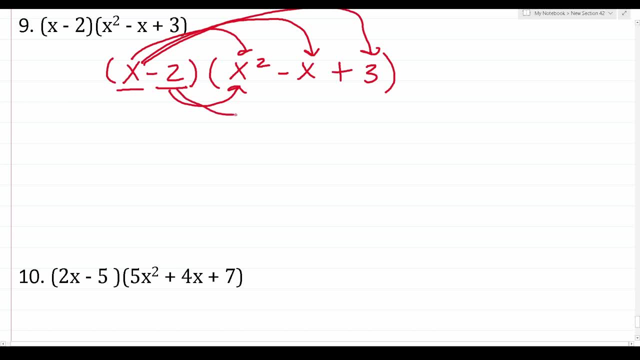 And we're going to take this negative 2 and distribute it here, here and here. Let's go ahead and work on doing that Again. to start, we have x times x squared, So that's again x times x squared. 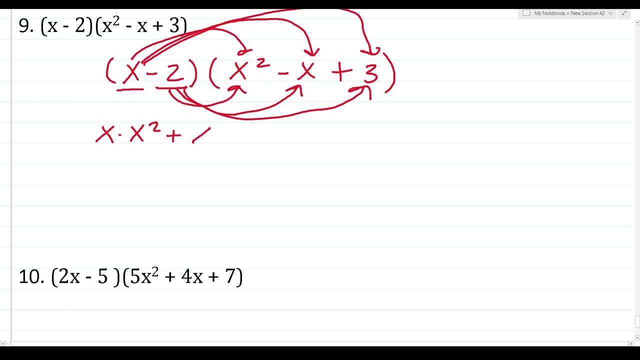 Then we have x times negative x. So this is plus x times negative x. Then we have x times 3.. So this is plus x times 3.. And then we're moving on to our negative 2. So we have minus 2 times x squared. 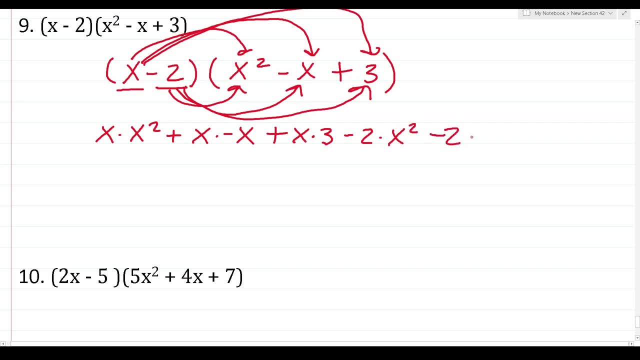 And then we have minus 2 times negative x, And then, finally, we have minus 2 times positive 3.. Let's go ahead and simplify this now Again, we can use the product rule here, So this becomes x to the 1 plus 2.. 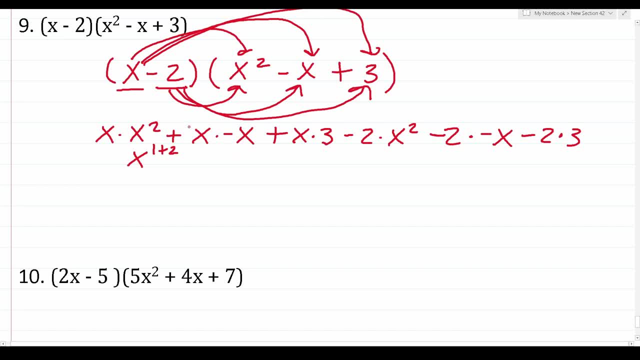 And then we can use the product rule here. But that said, we have an implied 1 here, So this is 1 times negative 1.. So this is going to be negative, And then this is just x 1 plus 1.. 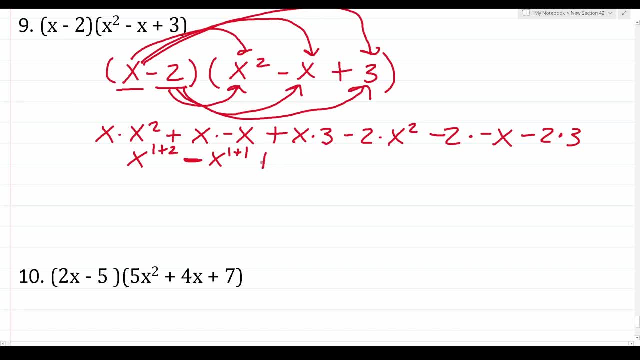 Right here we just have x times 3, which is just 3x, So this is plus 3x. Right here we have negative 2 times x squared, So that's negative 2x squared. Right here we have negative 2 times negative x. 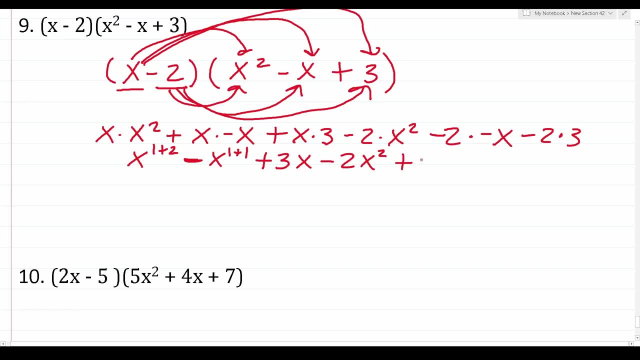 Negative times: a negative is a positive, So that's going to be plus 2x. And then, finally, we have negative 2 times positive, 3.. And negative times: a positive is a negative, So that's going to be negative 6.. 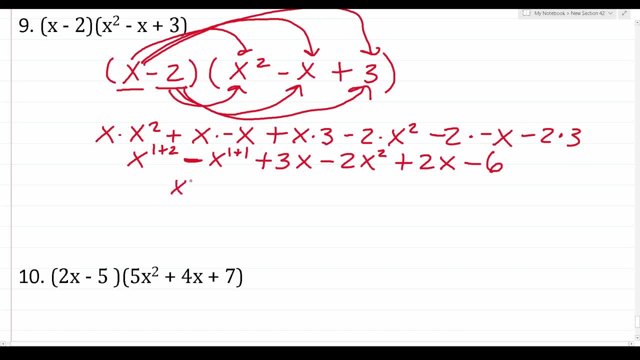 All right, Let's go ahead and keep cleaning this up. So we have x to the 3rd minus x squared plus 3x minus 2x squared plus 2x minus 6.. Let's combine like terms: x to the 3rd doesn't have anything, we can combine it with. 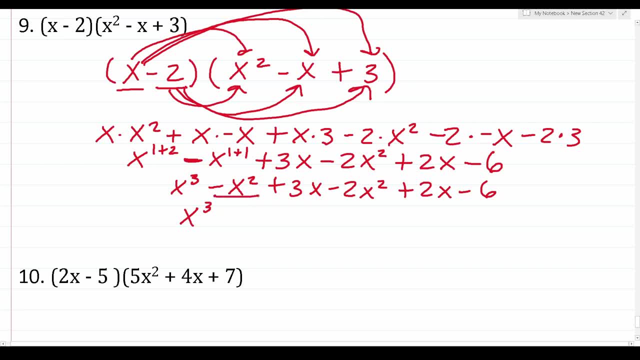 But that said, this negative x squared can be combined with this negative 2x squared to become negative 2x squared. So that's going to become negative 3x squared Again. yesterday I uploaded a video regarding adding polynomials. 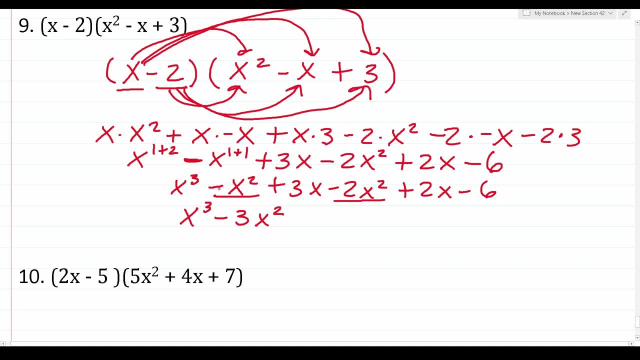 So if you need to watch that, you can go ahead and do so. So we've taken care of that. Let's just go ahead and put a line through it to indicate that we've done so. Now we have 3x and 2x, which are like terms. 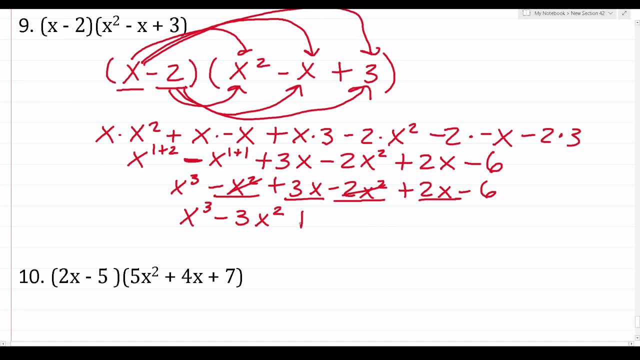 So we can go ahead and add those such that it becomes plus 5x And then we just have minus 6.. And, as you can see, we expressed this, So we're going to write this one such that the highest order polynomial comes first. 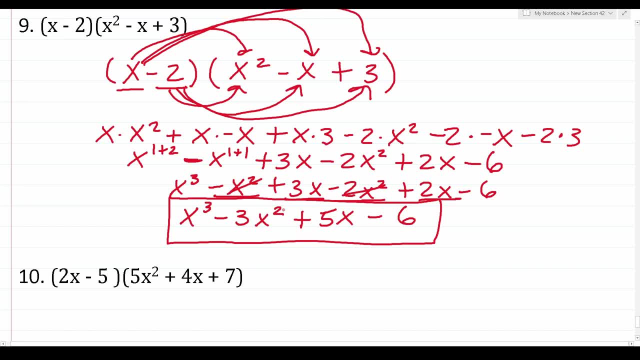 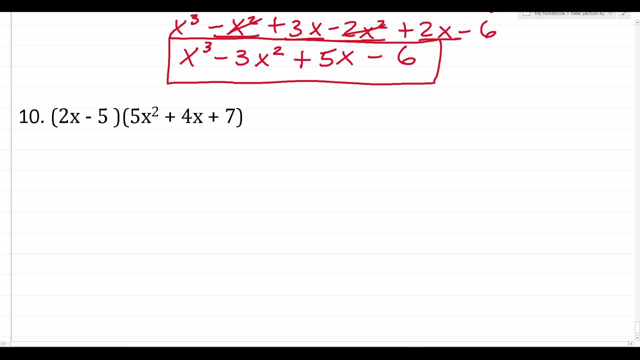 followed by the next exponent, next, and so on and so forth. So that's that one, All right. So for number 10, I'm not going to work everything out, I'm just going to go pretty much straight to the answer to show you that you can get. 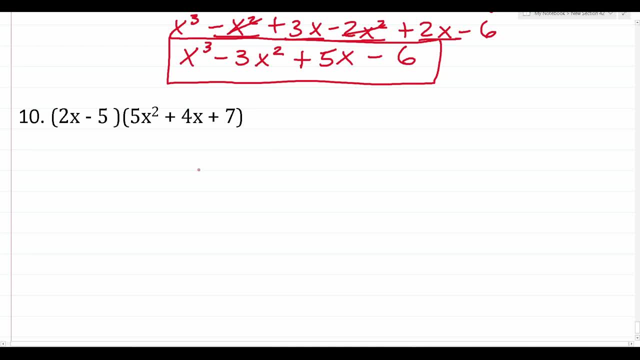 good enough at these, such that these problems are very easy. So, that said, I will write it out. So if you're viewing this on a mobile device, you can see the question better. Again, we have 2x minus 5.. 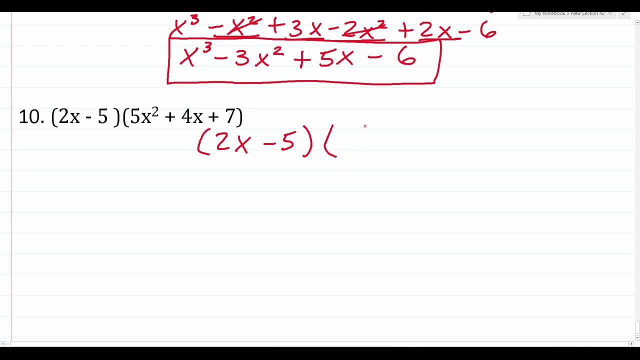 And my pen is starting to act up here- Times 5x squared plus 4x plus 7.. Again, we're going to use the distributive property, which means we're going to take this first term and multiply it by all these terms. 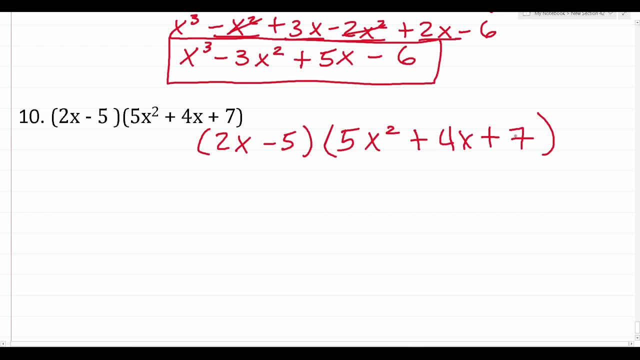 And we're going to come back And we're going to take this first term and multiply it by all these terms, And we're going to take this second term and multiply it by all these terms. I know I've been drawing lines in an effort to show you how to do that. 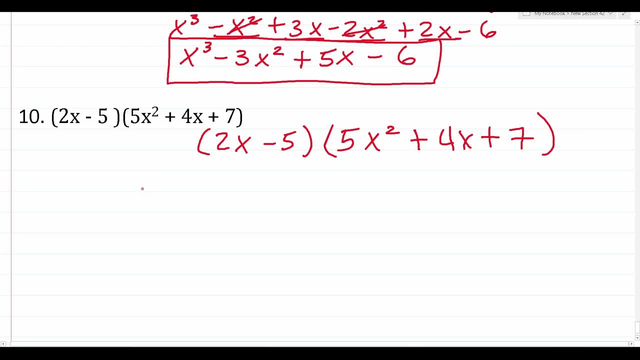 But again, I'm working this one out as if I was taking the test. So to start, I got 2x times 5x squared, So I know that's going to be 10 for my coefficient, And then x to the 1 times x squared is going to be x to the third. 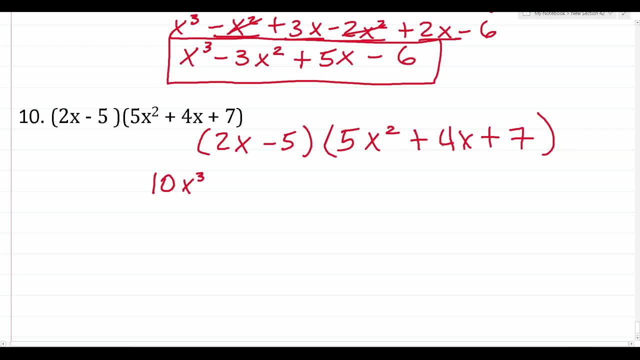 Let's move on. We have. We have 2x times 4x, So that's going to become plus 8x squared. And then we have 2x times 7. So that's going to become 14x. 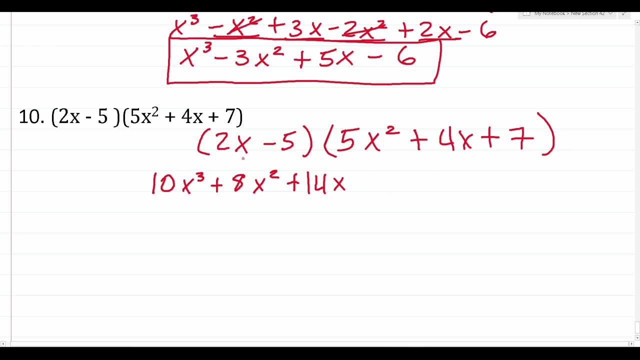 My pen is starting to run out of battery here, So bear with me. So I just did 2x times all these terms. Let's go back and work on this negative 5 now. So we're going to multiply coefficients of negative 5 and positive 5.. 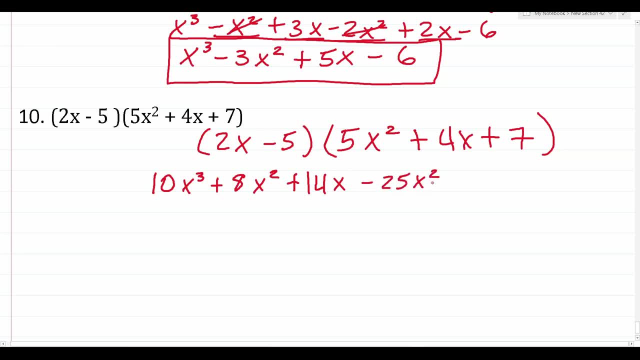 So that's going to be Minus 25x squared. And then we have negative 5 times positive 4, which is negative 20.. And there's nothing to do with the x's there except to tack it on. And then we have negative 5 and positive 7,, which is negative 35.. 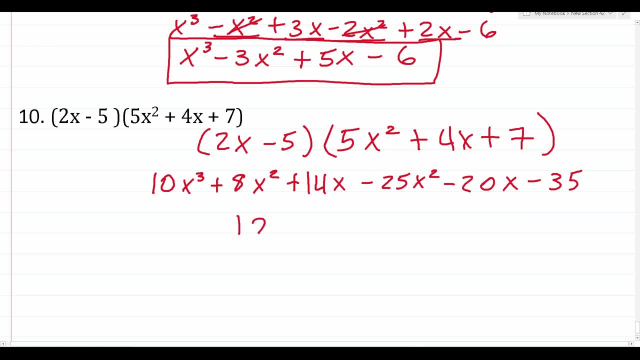 Let's go ahead and see if we got some like terms we can combine. We have 10x to the third, Nothing to combine that with. That said, we have 8x squared and negative 25x squared, So that's the same thing as 25 minus 8, which is going to be 5 minus 8.. 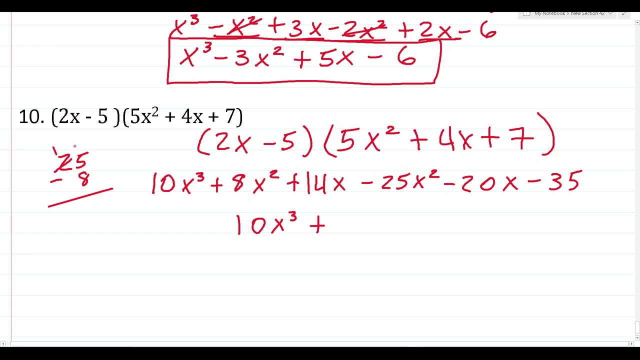 We can't do, We have to borrow. This becomes 1.. This becomes 15.. 15 minus 8 is 7. And 1 minus nothing is 1.. So this is not plus, And let me get my eraser here. 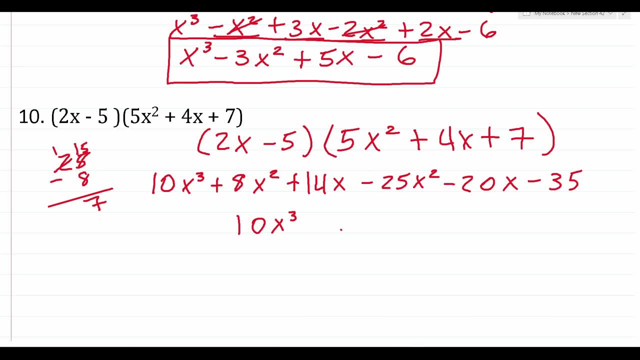 This is not plus, This is Minus 17x squared. Again, I just took this 8x squared and combined it with this negative 25x squared, which is negative 17x squared, And then I have this 14x and this negative 20x.